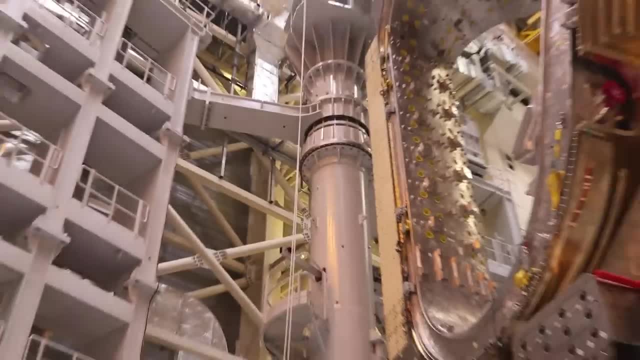 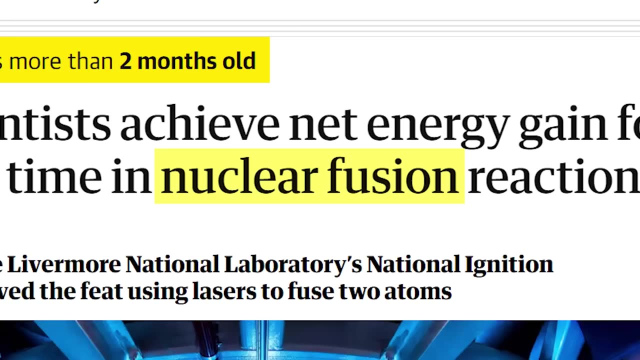 I went to a place history is being made the largest nuclear fusion reactor in the world. Wow, it's so huge. Everywhere you look, nuclear fusion is the talk of the town. Nuclear fusion- A nuclear fusion. Nuclear fusion, Nuclear fusion. 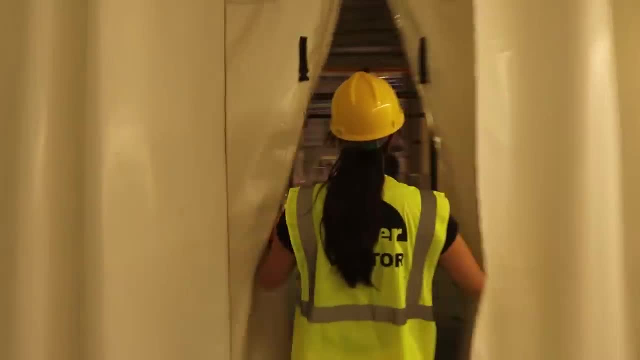 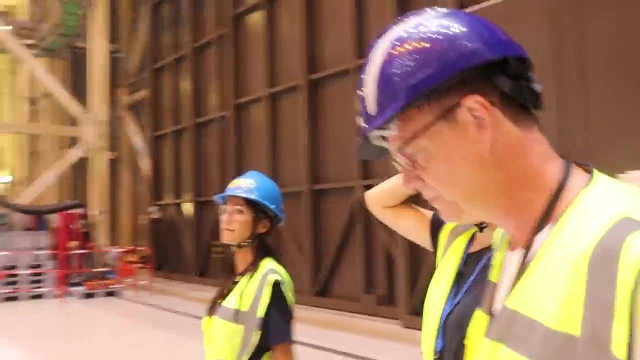 I just had to find out what all the hype was about and I thought: what better way than to go to the center of where it's all happening and, of course, bring you guys along? I want to learn as much about fusion as I can today. 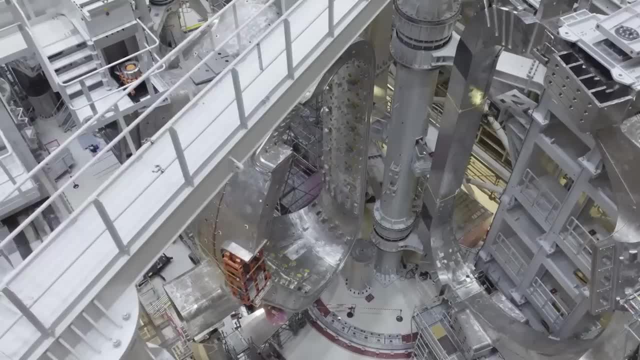 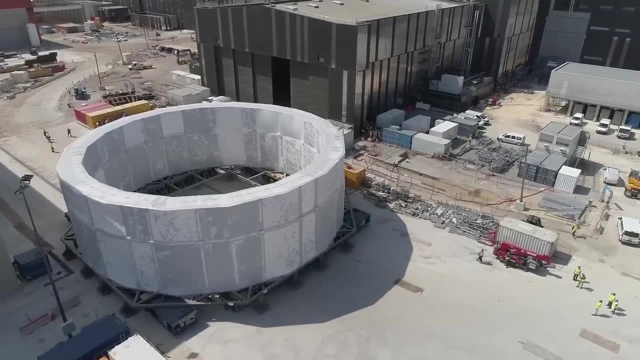 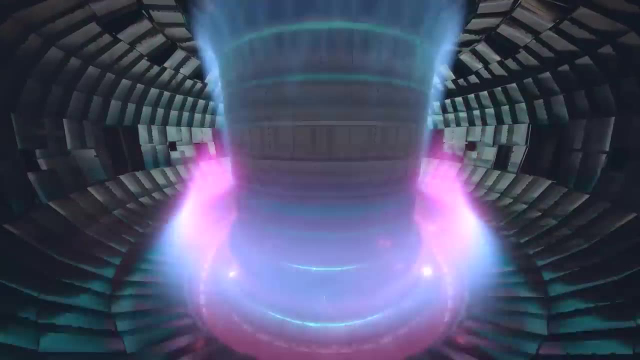 This is ITER, an International Thermonuclear Experimental Reactor. It's been described as the most expensive science experiment of all time and the most complicated engineering project in human history. It aims to bring nuclear fusion, the process which powers the stars, down here on Earth. 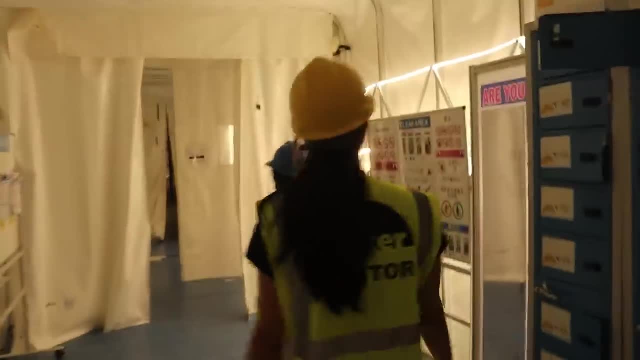 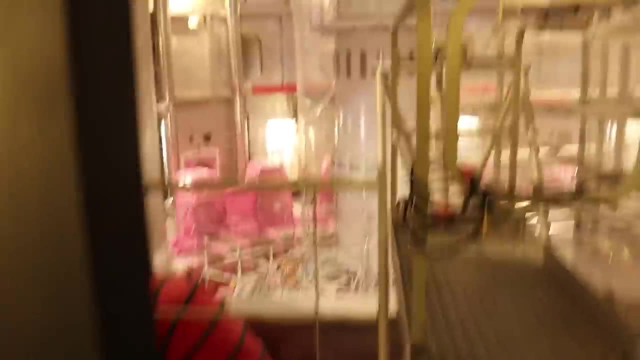 But what really is nuclear fusion? What is happening behind the doors of this $20 billion megaproject? When will it be ready, and is it really all it's hyped up to be? This is not a technology. This is a technology that will solve the climate problem. 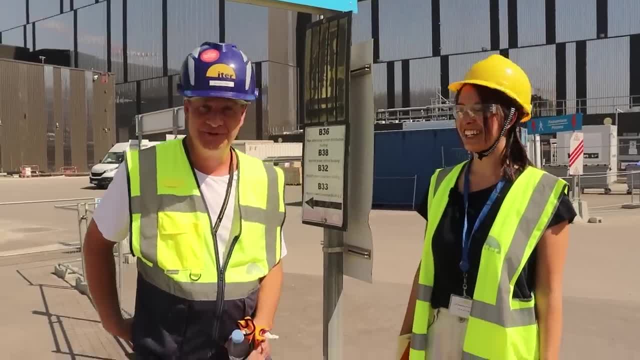 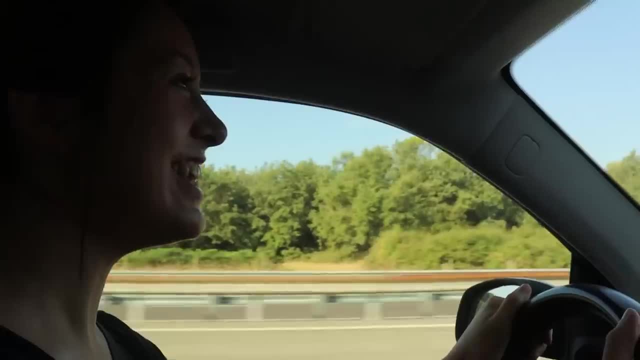 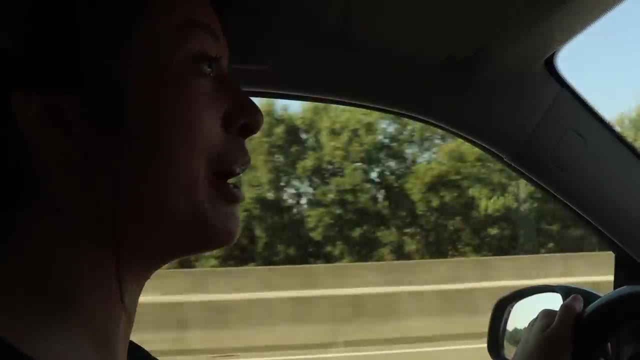 Today we're going to find answers, meet some incredible people and see some extraordinary things. Let's start from the beginning. Today we're going to the world's biggest nuclear fusion reactor. It's located in the south of France, in a town that I can't pronounce. 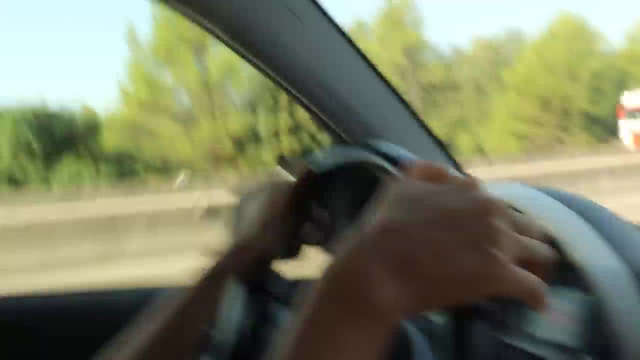 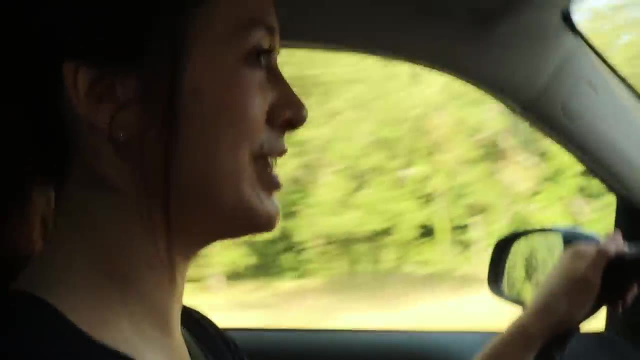 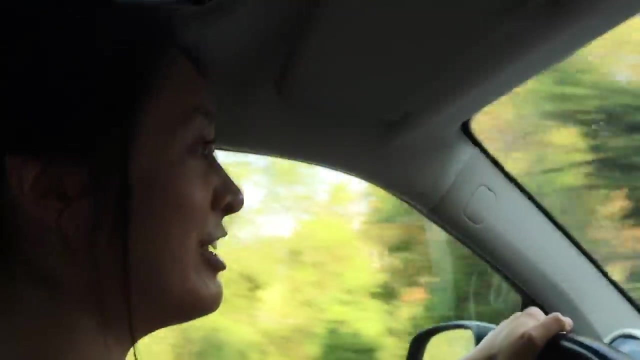 Simon, can you pronounce it? for us It's a bit like endurance, Cool. So currently what I know about nuclear fusion is that it's the, It's the process that powers the sun. If we could harness nuclear fusion on Earth in a sustainable way, it would be completely revolutionary. I know it's very difficult to achieve engineering-wise. Yeah, hopefully we can one day achieve it, because that would be cool. That was about the extent of my knowledge I'd heard. harnessing the power of nuclear fusion would be revolutionary. 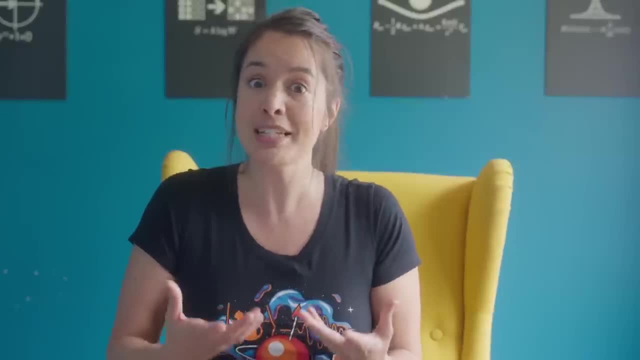 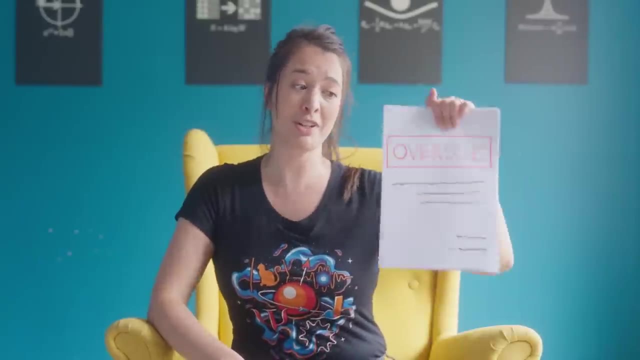 but I didn't know why. What could justify forking out $20 billion to bring it down to Earth? Well, life's conveniences come at a cost, And not just what shows up on your electricity bill. Our societies run on electricity. 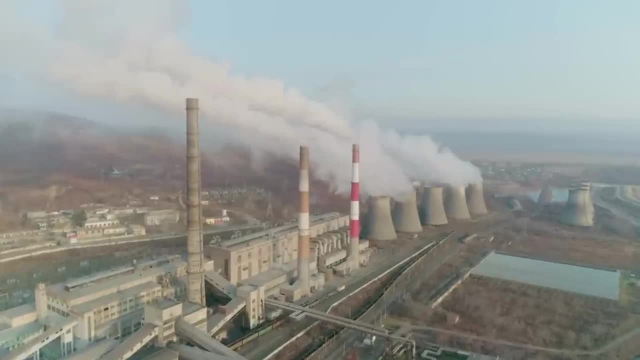 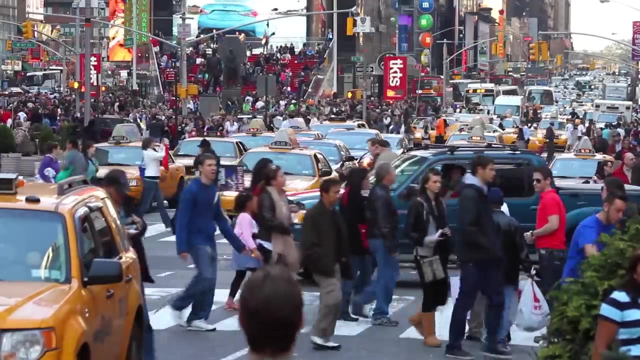 But where does it come from? Most of our power comes from fossil fuels like coal, gas and oil, which we dig up from the Earth's crust. But fossil fuels are finite and, with the population growing and demand increasing, it's looking like they may run out sooner rather than later. Prices are steadily rising And about 1 in 10 people don't have access to electricity. What's more is that burning these fossil fuels is harming our planet. They release toxic and greenhouse gases which cause global warming and air pollution. It's like the mess after a party that no one wants to clean up. 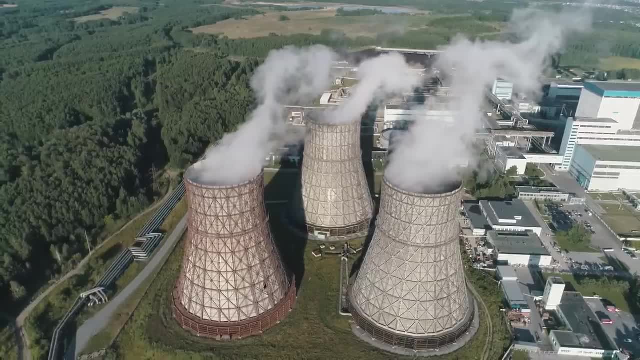 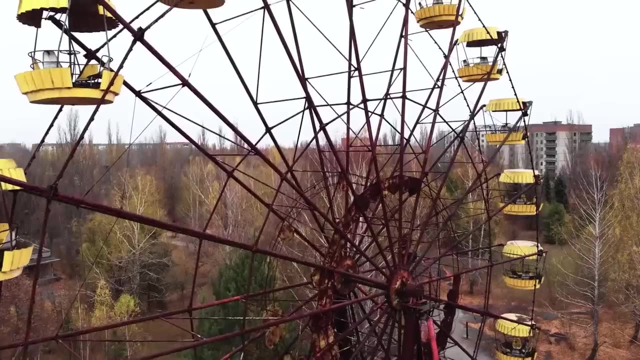 The other main way we turn energy into electricity is through nuclear fission in power plants. But this has problems too. It creates nuclear wastes which last thousands of years, And accidents can be extremely dangerous- Think nuclear meltdowns. A new source of energy is the nuclear power plant. A new source of energy is desperately needed. But what Nuclear fusion solves basically all of these problems. It's generated from two abundant resources- seawater and lithium, So there's no risk of them running out any time soon. The reaction creates roughly 4 million times more energy than fossil fuels. 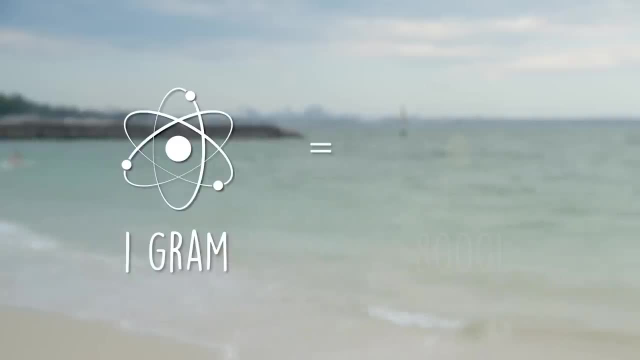 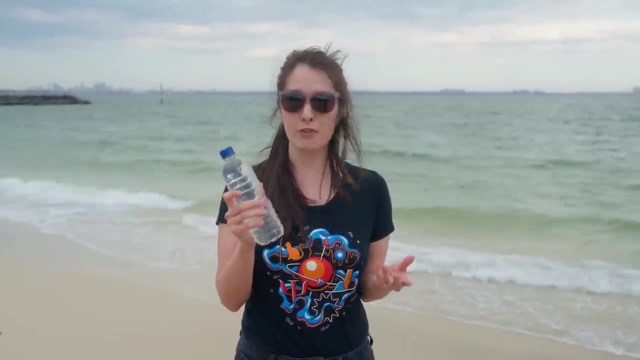 One gram of nuclear fusion fuel produces the energy equivalent to 8,000 litres of heating oil. This water bottle full of seawater plus one gram of lithium could provide electricity to a family of four for a whole year. Everyone would have access to cheap and abundant electricity. It produces virtually no harmful gases or air pollutants And there's no long-lived nuclear waste. There's also no risk of a meltdown. It's safe and environmentally friendly. Nuclear fusion on commercial scales could potentially revolutionise energy consumption. That is why we're forking out 20 billion dollars to crack it. It's considered by many to be the next step in humanity. So what's the catch? It's really hard, Really hard. The fuels need to be heated to temperatures 10 times hotter than the sun. That's pretty hot. This poses enormous engineering challenges. 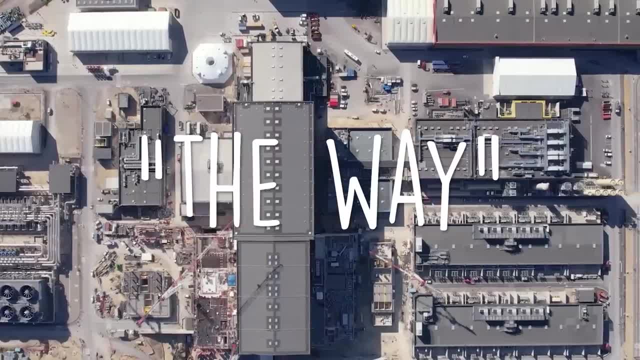 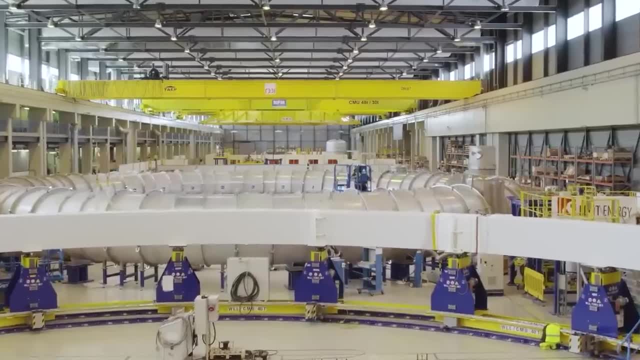 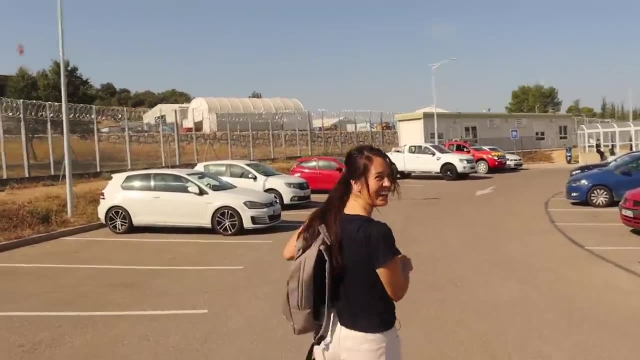 But ITER, which means The Way in Latin, is taking on this mammoth challenge. Their aim is to develop a fusion reactor on the scale of a power plant and in doing so, showcase the feasibility of commercial nuclear fusion. When we arrived, we were met by 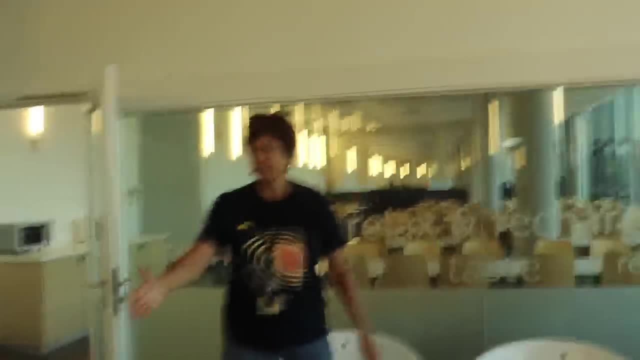 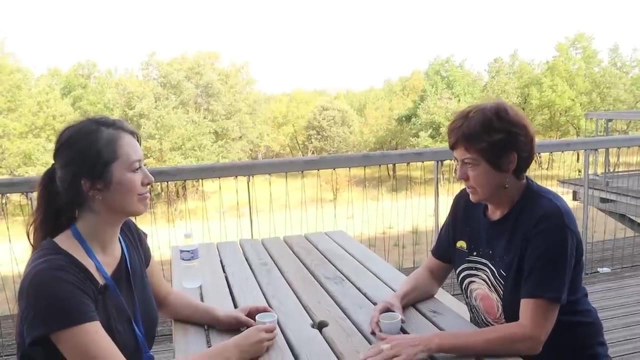 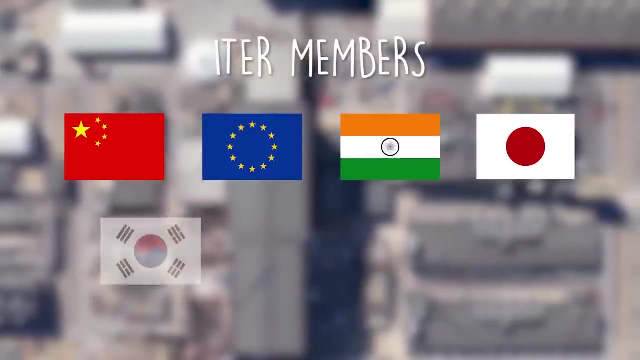 Julie and Sabina. So hi, Jade, welcome to ITER. Hi, I'm Jade, nice to meet you, Jane, Who told us the backstory and goals of ITER. ITER is currently the largest international scientific corporation in the world. Seven members: China, the European Union, India, Japan, Korea, Russia and the United States. 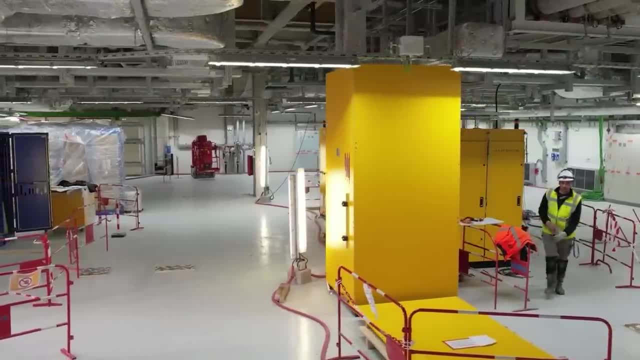 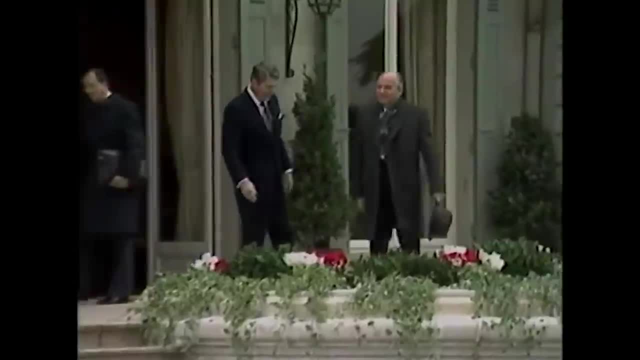 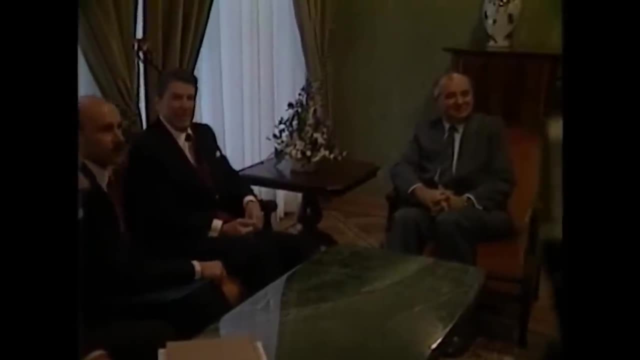 So there was this energy summit in the United States. So there was this energy summit in Geneva in 1985, where Ronald Reagan and Gorbachev met and decided to launch this huge international collaboration with the aim of bringing a clean energy for peaceful purposes. 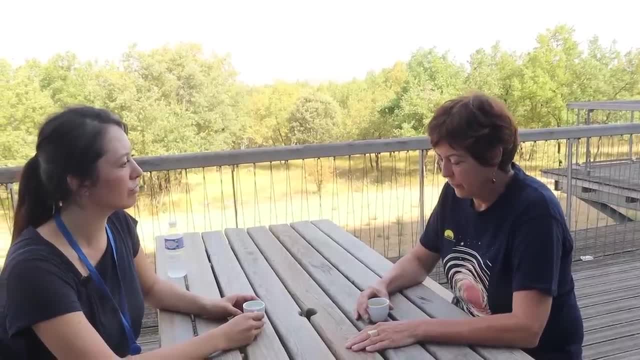 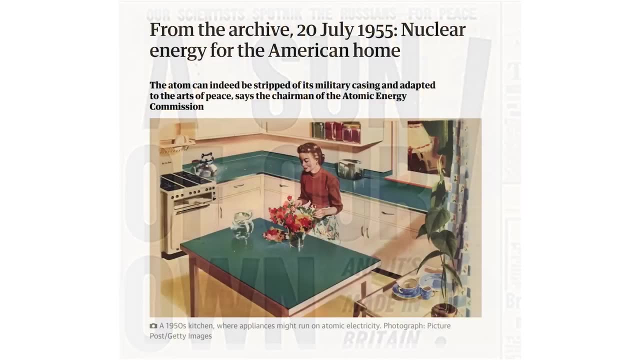 The goal of our quest is to prove that we can produce net energy with fusing atoms. Nuclear fusion isn't a new science. It's been around since the 50s. The tricky part is getting more energy out than you put in. Nuclear fusion isn't a new science. It's been around since the 50s. 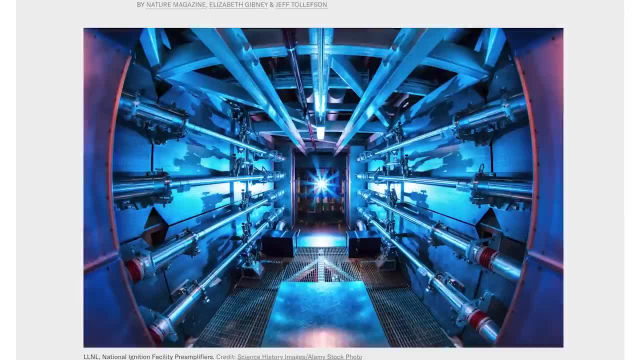 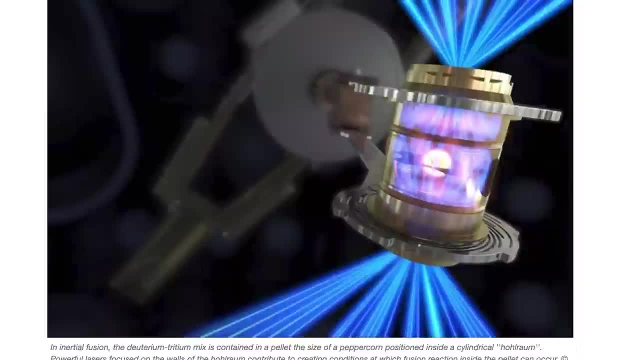 This has only ever been achieved once in fusion history. late last year, at the National Ignition Facility, Scientists put in two megajoules of power and got out three megajoules- a gain of 1.5 in fusion torque. 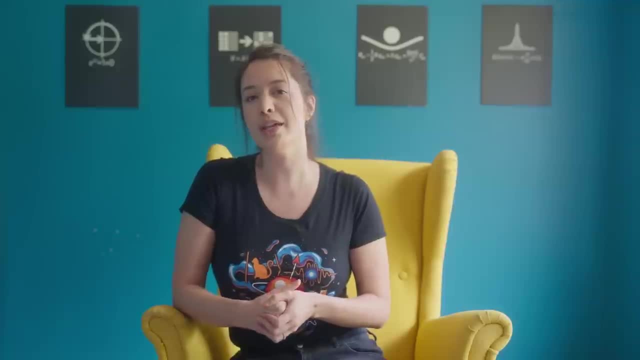 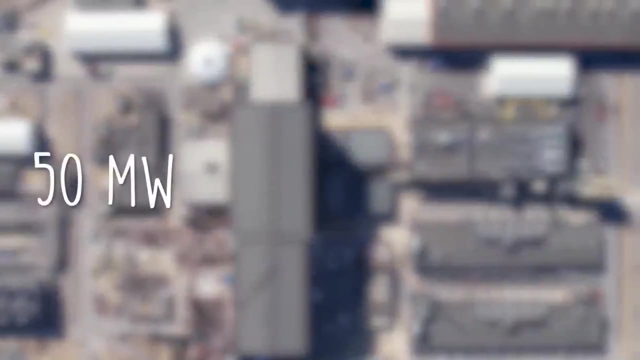 While it was definitely a scientific feat, the energy output was only about enough to boil water for 30 cups of coffee. ITER is aiming for much higher energy gains: an input of 50 megawatts of thermal power and an output of 500 megawatts of fusion power. 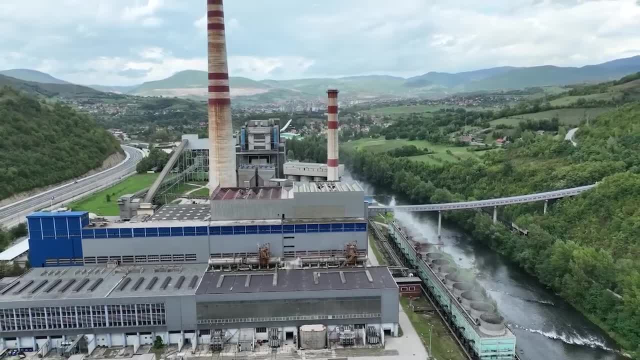 an input of 50 megawatts of thermal power and an output of 500 megawatts of fusion power, a gain of 10.. For context, 500 megawatts is comparable to the average nameplate capacity of a coal-fired plant. 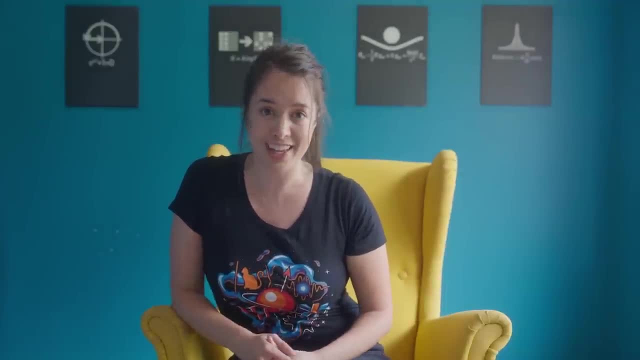 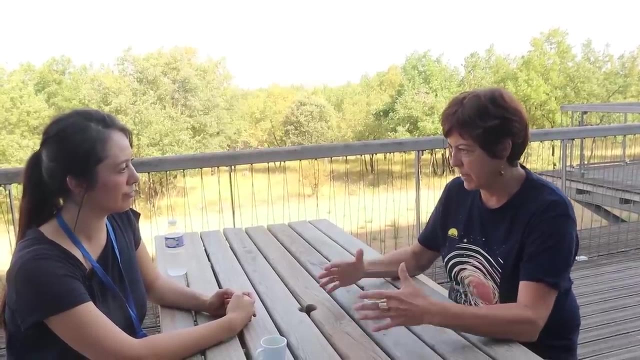 There's a pretty big gap between that and 30 cups of coffee. So how is ITER going to achieve this? The core and the heart of ITER is certainly the machine tokamak machine that we are building here. When it comes to nuclear fusion, size is important. 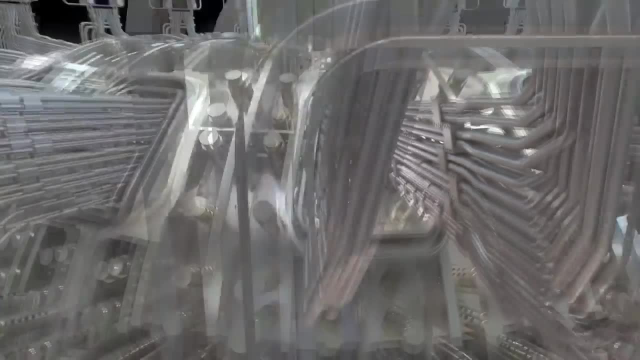 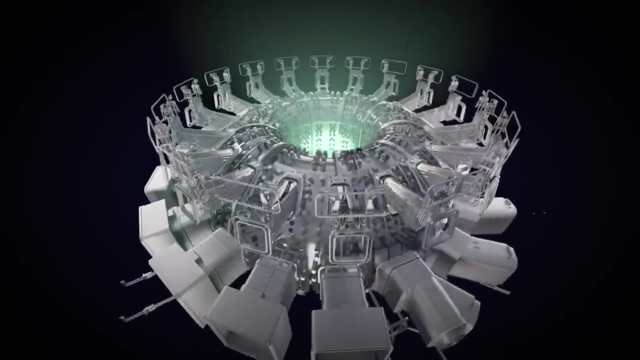 No other nuclear fusion device on Earth even comes close to the size of the ITER tokamak- an important subject. The main subtlety is that ITER will not actually produce electricity. It's an experimental reactor designed to perfect the technologies needed for a real fusion reactor. 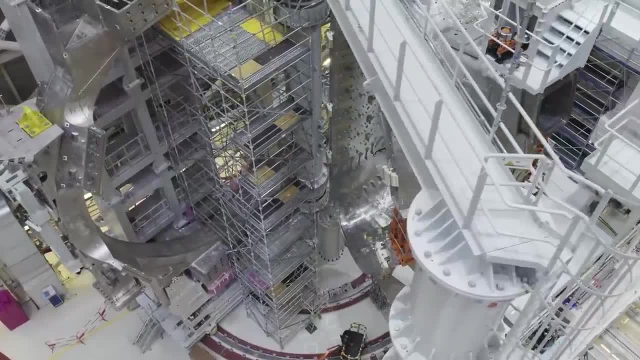 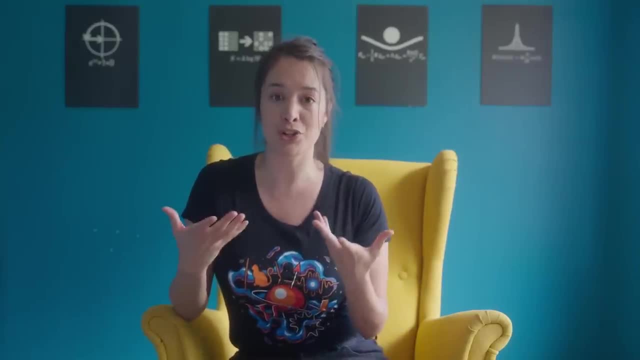 A lot of what they're doing here, from the engineering to the science to the collaboration style, has never been done before. If all goes according to plan, it'll be the last step before a real commercial fusion reactor, one that does produce electricity. 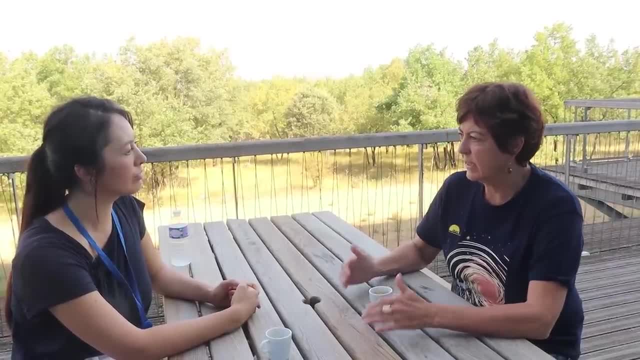 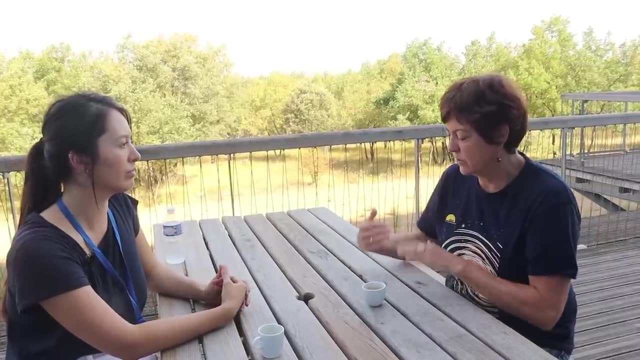 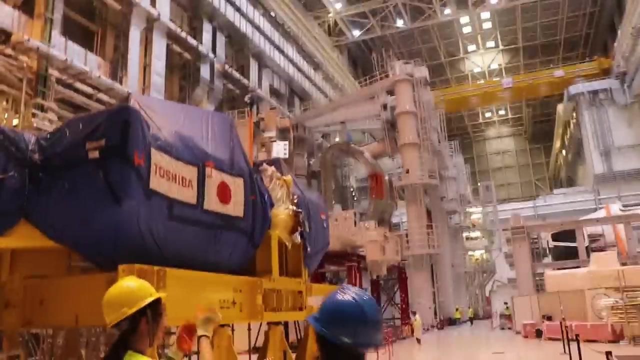 But the way we do it is a very peculiar way. We do it via in-kind contributions. That means the whole ITER machine is divided into different technologies, different components, and these components are distributed over all these partners. The reason behind these in-kind contributions is that it's teaching all the participating nations. 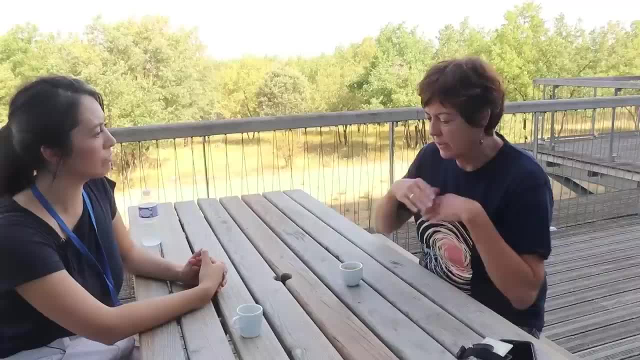 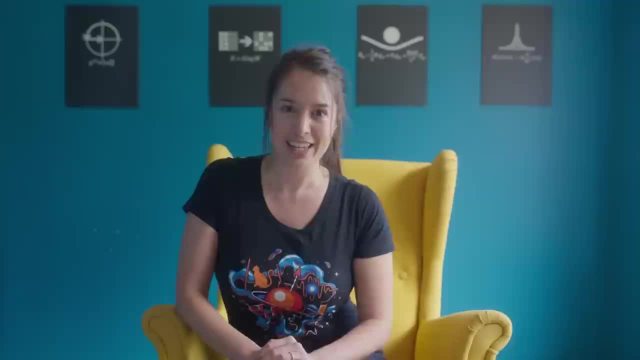 how to build and run a fully functioning fusion reactor And you can look at the machine. whatever component you look at, there are multiple nations working on one component. So after ITER is complete, they can start building their own fusion reactor. So after ITER is complete, they can start building their own fusion reactor. 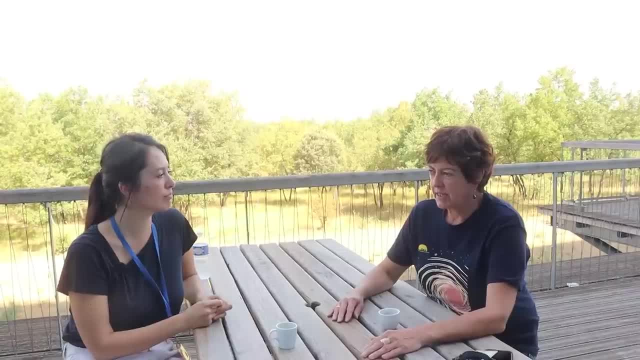 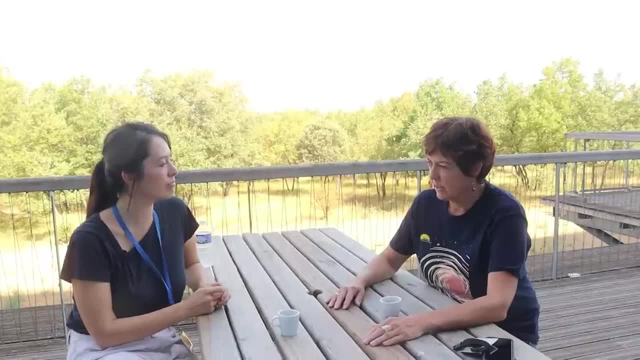 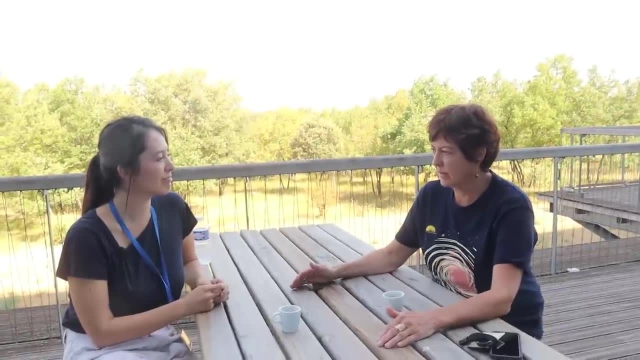 that have been at war with each other not so long ago, And this is amazing. And here we are sitting around the books of ITER and nuclear technology and we are doing this all together. So very often we talk about and we see ITER also as a peace project. 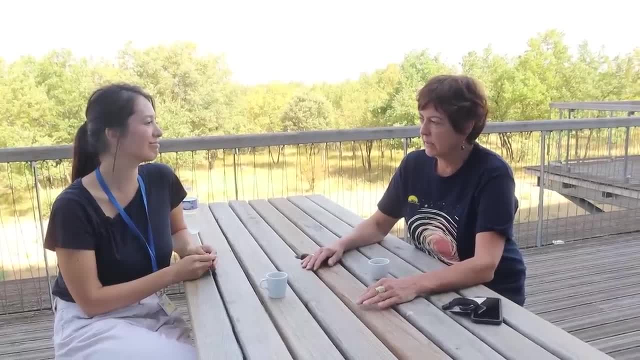 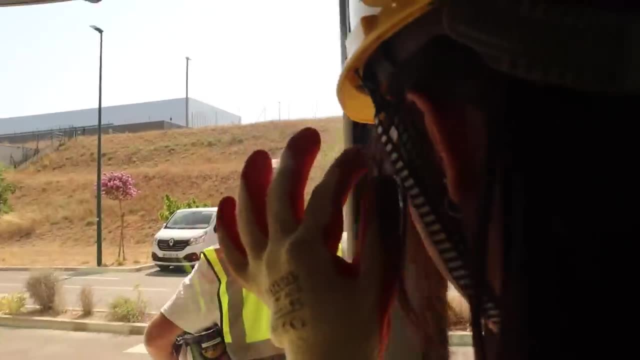 This, for me and for many of my colleagues, is the most amazing thing about ITER. This, for me and for many of my colleagues, is the most amazing thing about ITER. This is Richard Pitts, one of the senior physicists here at ITER. 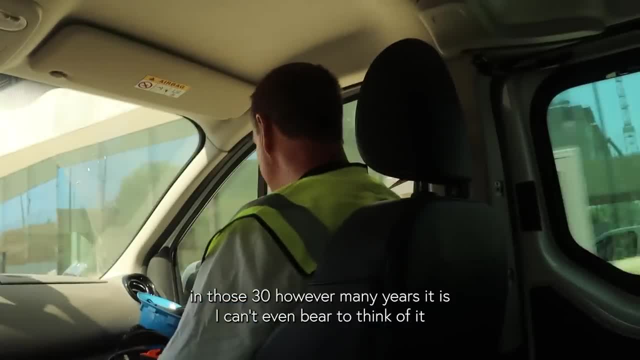 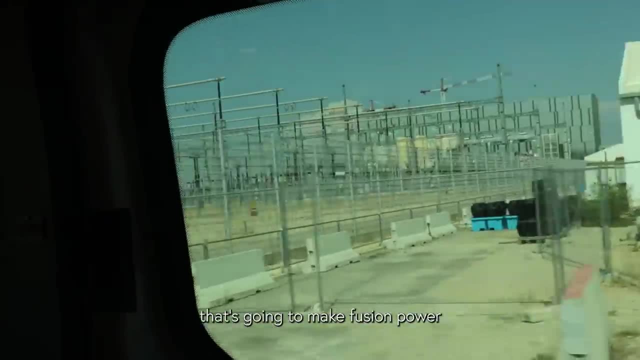 This is Richard Pitts, one of the senior physicists here at ITER, So I've worked on practically all of these devices worldwide in the last 30, however many years it is, I can't even bear to think about it. If you really want to be involved in the one that's going to make fusion power, then this is it. 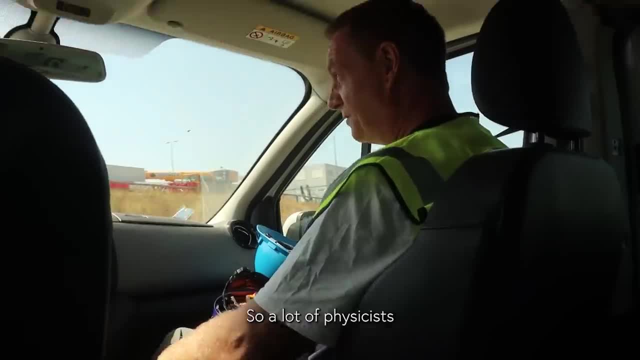 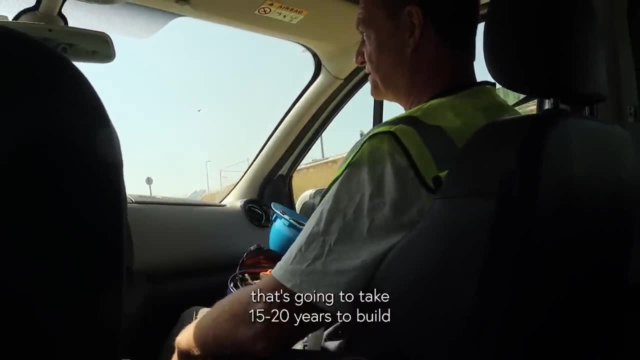 The only problem is it's a very, very long project, And so a lot of physicists, a lot of my colleagues in the physics community, they're just not prepared to sit on a project that's going to take 15 to 20 years to build. 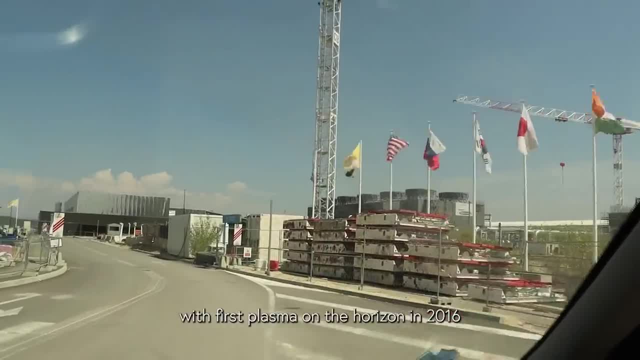 And so a lot of physicists, a lot of my colleagues in the physics community. they're just not prepared to sit on a project that's going to take 15 to 20 years to build. I came here in 2008 with first plasma on the horizon in 2016.. 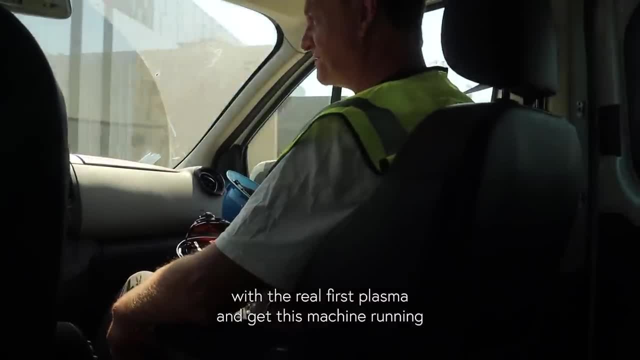 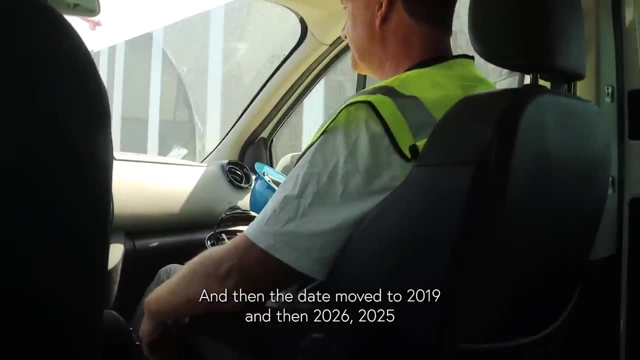 I thought, OK, I'll do 10 years roughly, and then we get to play with the real first plasmas and get this machine right. And then the date moved to 2019, and then to 2026, 25.. 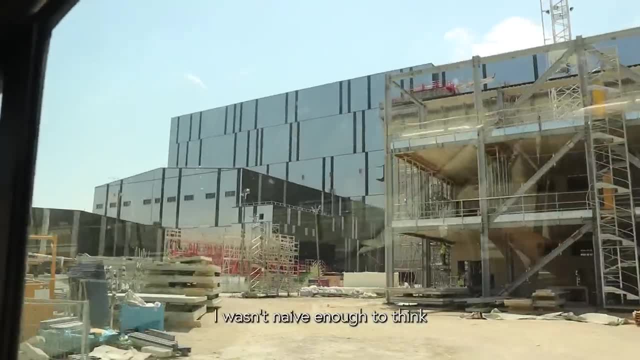 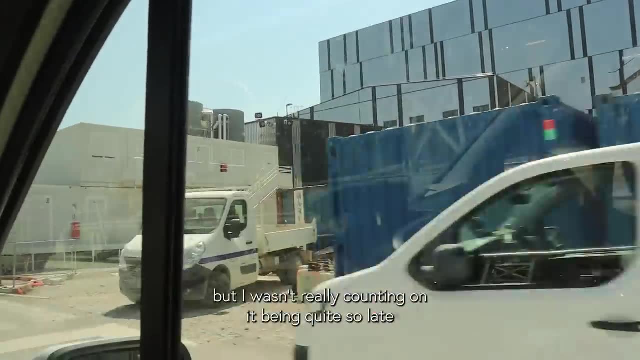 And now it will be again much later than that. I was naive enough to think that it would be really in 2016,, because I knew what kind of challenge this was, But I wasn't really counting on it being quite so late. So I will retire now, before. 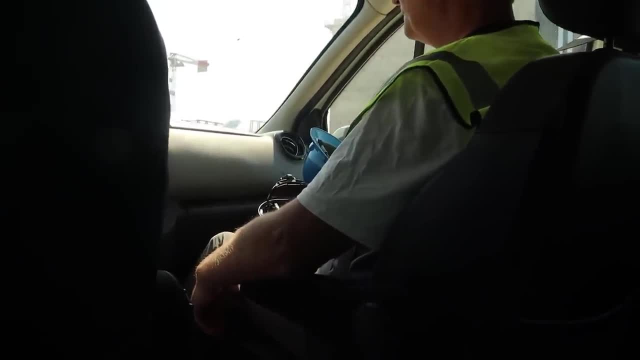 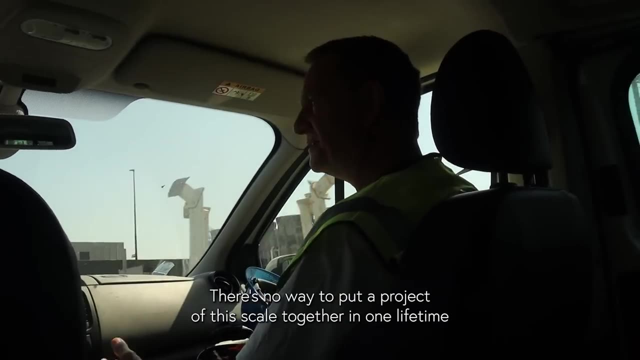 probably before any decent plasma is made. Oh, and how do you feel about that? Oh, I'm not very happy. You need people to get it ready so that other people can run it. There's no way to put a project of this scale together in one lifetime. 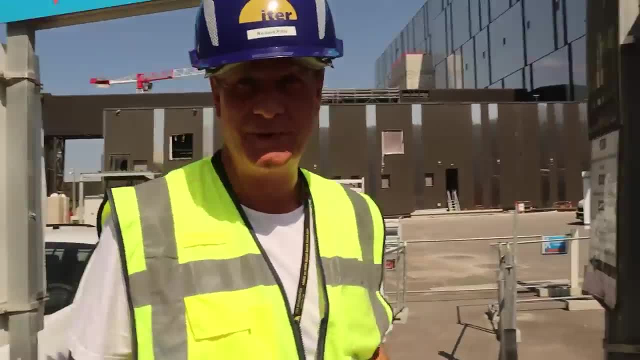 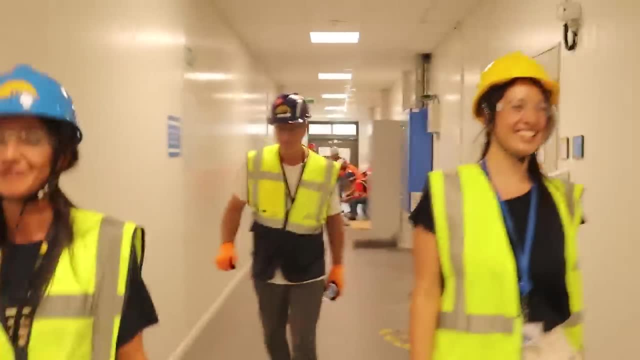 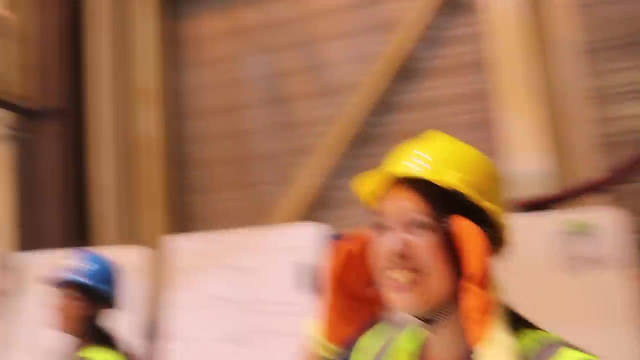 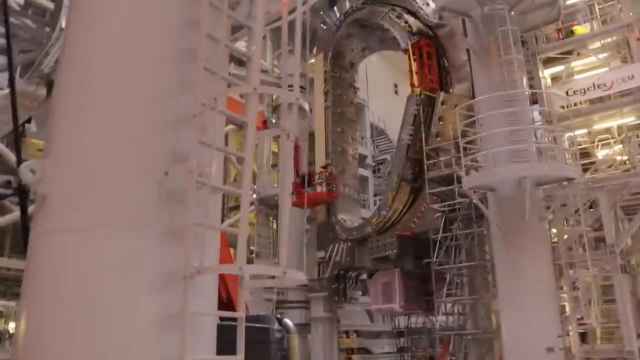 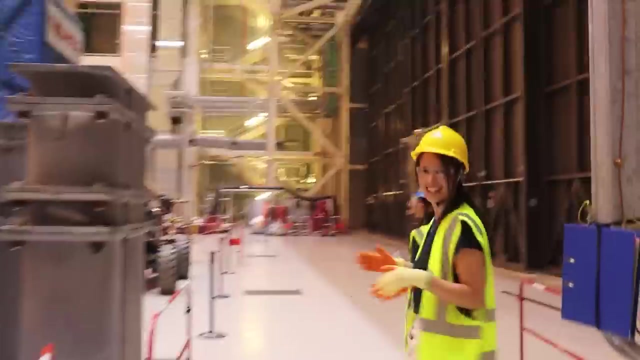 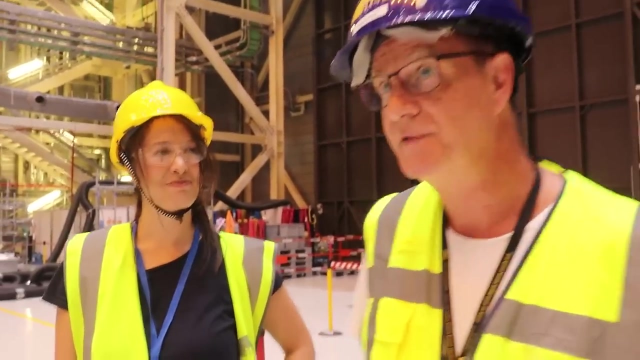 You can just see that bit of concrete sticking out. That's the start of the Tokamak building itself, which is a full nuclear grade seismic building. Wow, it's so huge. We'll start with that. What is nuclear fusion? Nuclear fusion, as you probably know, is the source of energy which powers the stars. 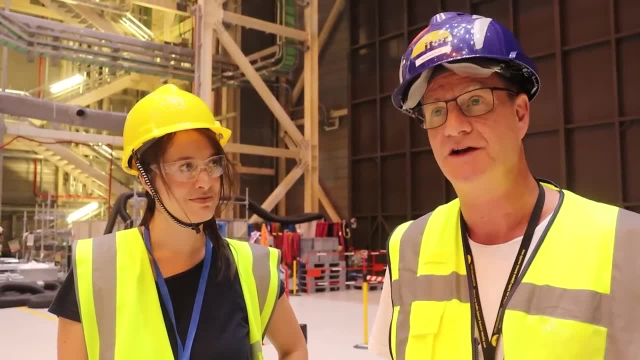 It is the opposite process to nuclear fission. Instead, it's a nuclear fusion. Instead of taking one large nucleus and splitting it apart with a neutron, you're taking two small ones, slamming them together as hard as you can and getting them to. 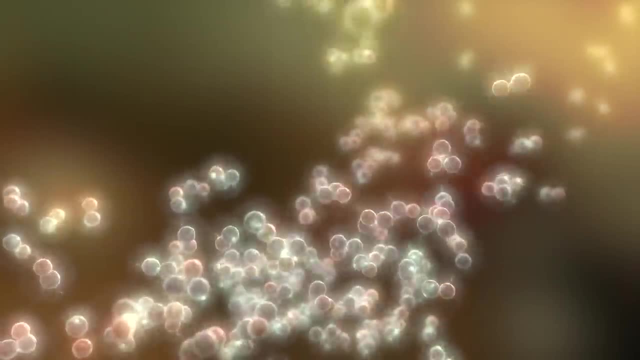 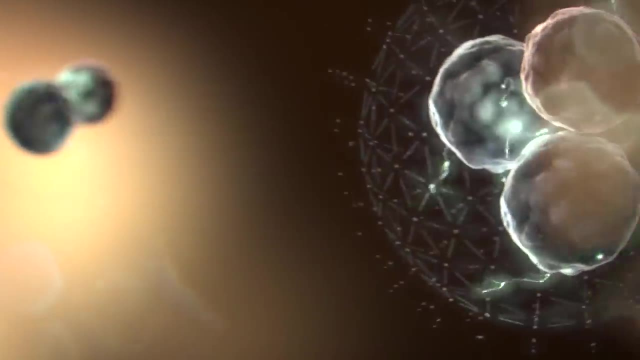 fuse, The resulting nucleus has less mass than the sum of the two original nuclei And, because of Einstein's, E equals mc squared, this releases a buttload of energy. The thing is, the conditions needed for these nuclei to fuse are not found naturally on Earth. 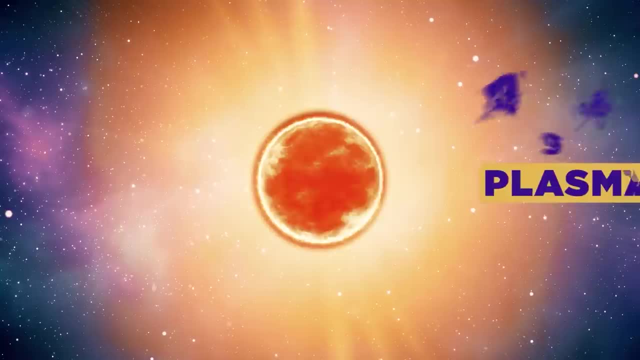 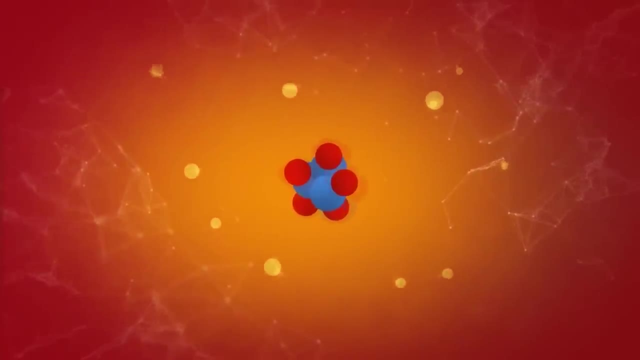 They're found in stars like our sun, which are made mostly of plasma. Plasma is the force of gravity. Plasma is the force state of matter. When you heat up a gas to high enough temperatures, the electrons become so energetic that they break free from their nucleus. 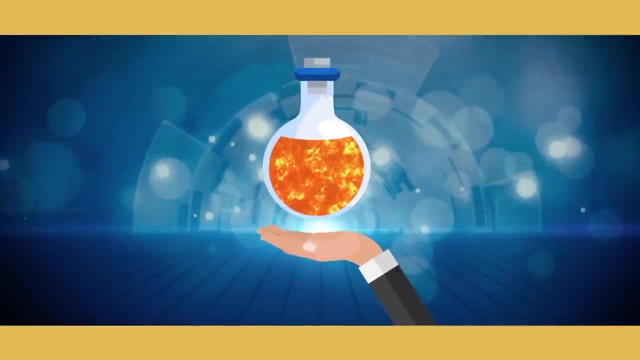 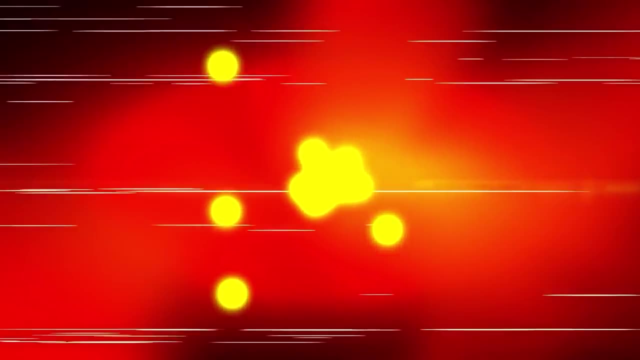 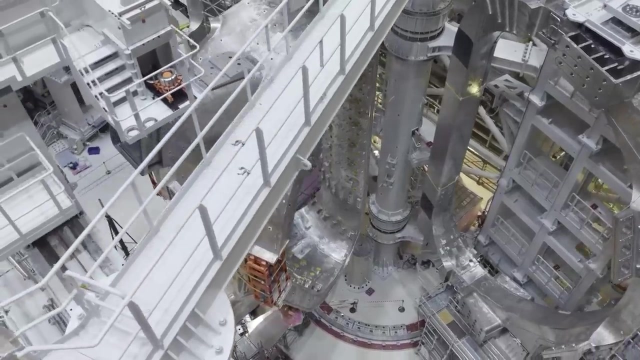 The resulting electrically ionized, extremely hot, soupy thing is called plasma. High temperatures provoke high energy collisions and therefore fusion. So if we can create a sustained plasma here on Earth, we should be all set to make nuclear fusion. That's exactly what ITER aims to do: create large amounts of plasma with the Tokamak. 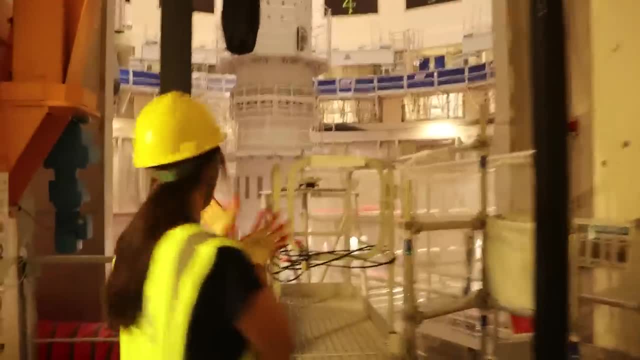 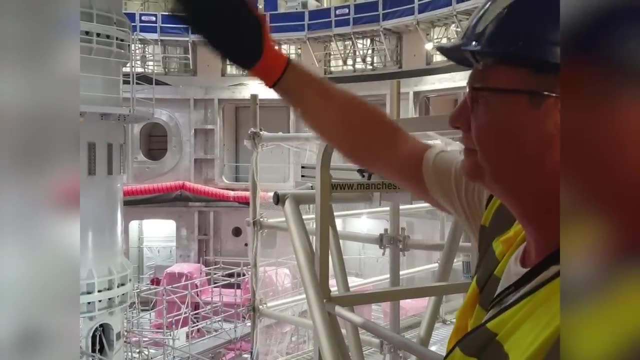 Okay, so this is where the Tokamak's going to be built, Correct, Is that right? This is where it is partially assembled. Partially assembled. Yeah, You're looking at the Tokamak pit. We are standing in the doorway, if you like, to the cryostat. 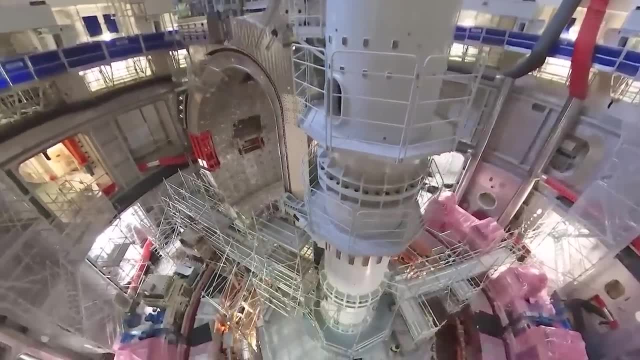 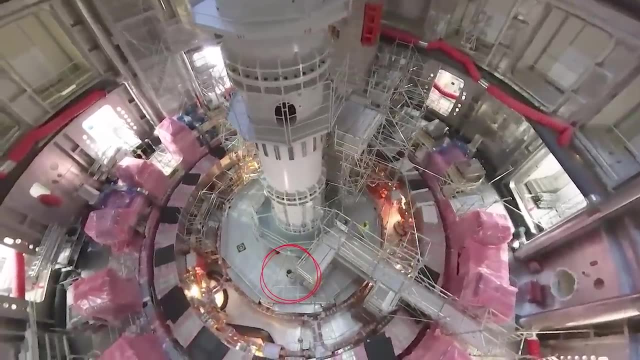 It was awkward to get a good shot of the Tokamak pit from where we were standing, so the kind folks at ITER gave me some drone footage to show you guys, There's a man for size comparison. It's going to be huge. 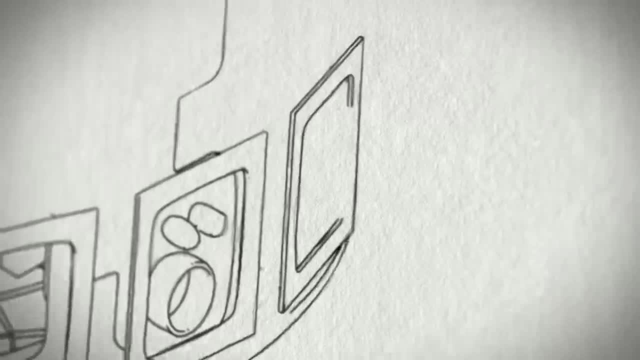 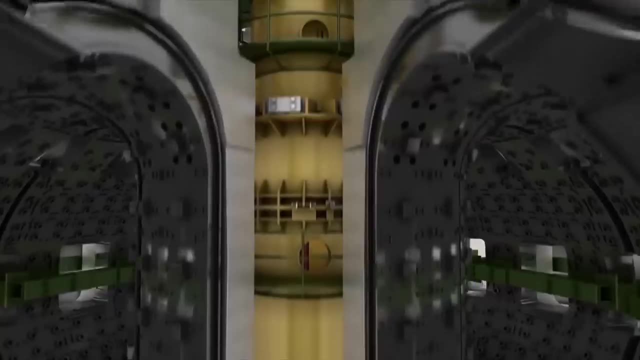 When it's complete, the ITER Tokamak will be 30 meters high and almost just one, And weigh 23,000 tons. That's more than most freight trains. It'll be made of around 1 million components and more than 10 million parts. 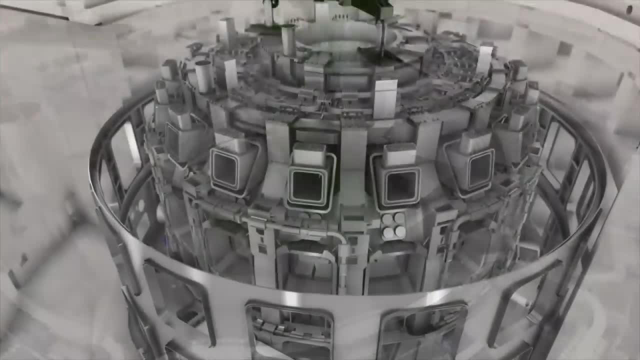 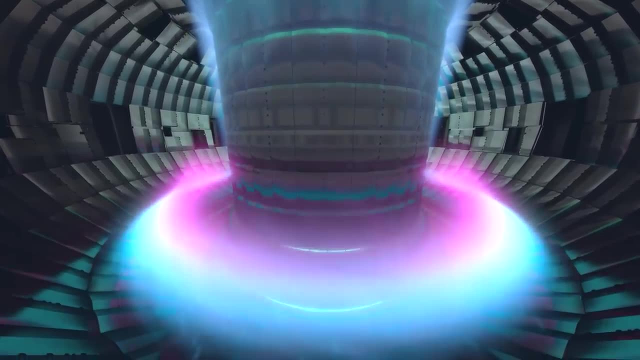 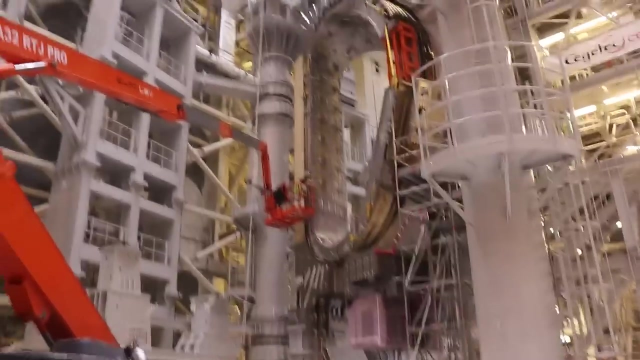 A giant, insanely complicated Lego puzzle. It'll hold a plasma volume of 840 cubic meters, roughly one-third of an Olympic-sized swimming pool and 10 times more than any existing Tokamak. You will put together nine sectors like this to make a ring, and we make the plasma. 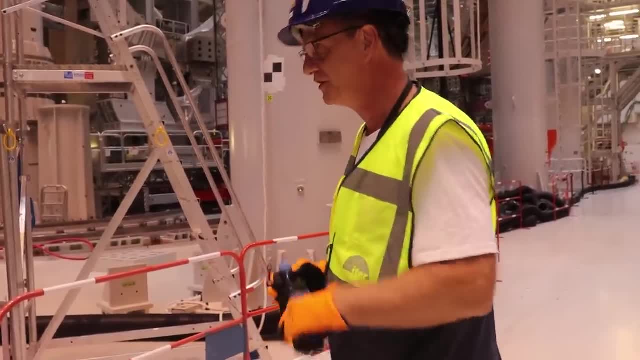 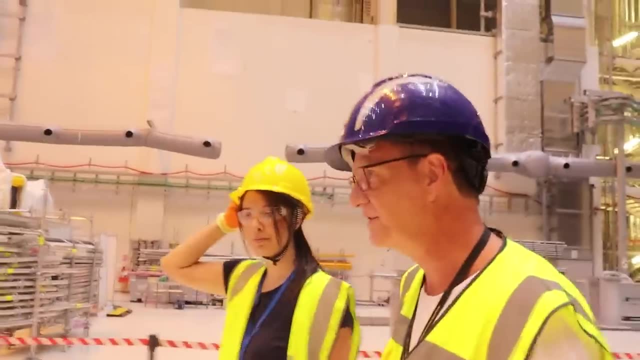 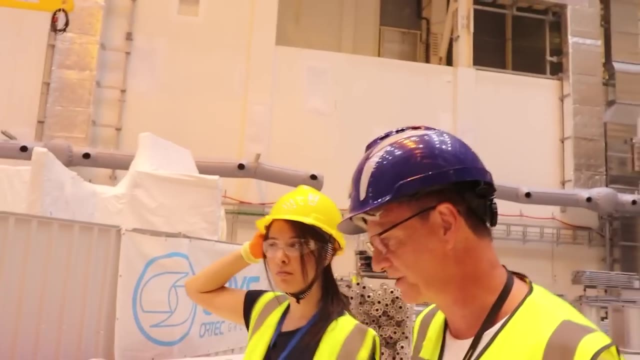 sit inside this toroidal ring And then we drive a current through it by injecting the current through a solenoid which is in the middle, And so you raise the temperature, and raise the temperature, push more and more current through the plasma and eventually you will reach conditions where fusion can start to occur. 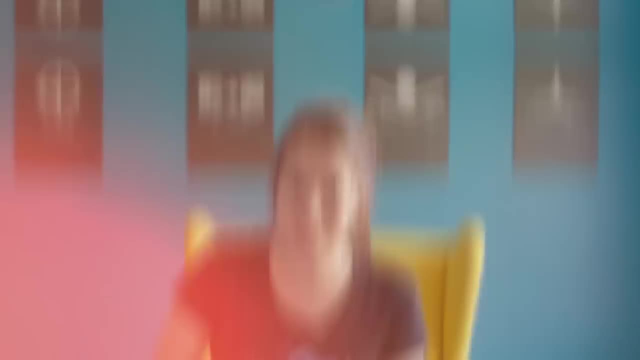 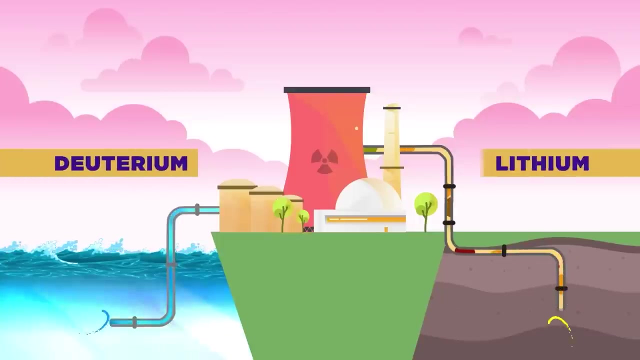 How will ITER generate temperatures that rival the sun's core? Deuterium and tritium are two isotopes of hydrogen and are the fuel for the fusion reactions. Deuterium is extracted from seawater And tritium is extracted from lithium. 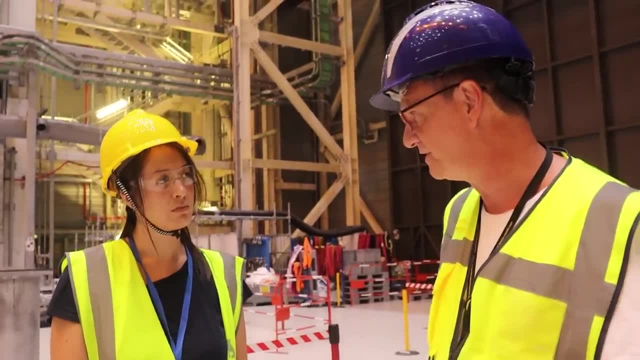 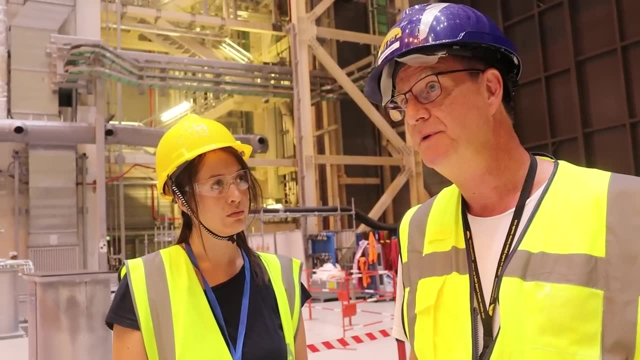 It turns out that the reactivity between deuterium and tritium is the highest at the lowest temperature of all possible fusion reactions, And so we use deuterium plus tritium. We put them together in a very large vacuum vessel, a bit of which you can see up there. 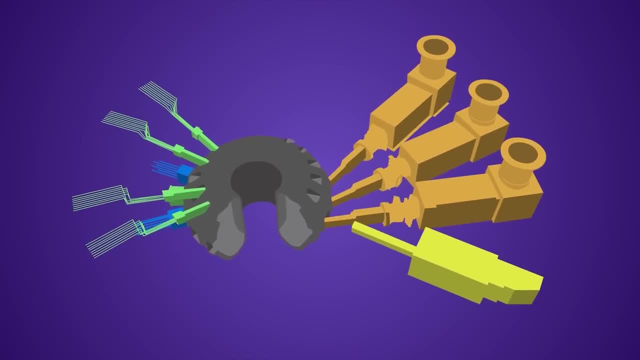 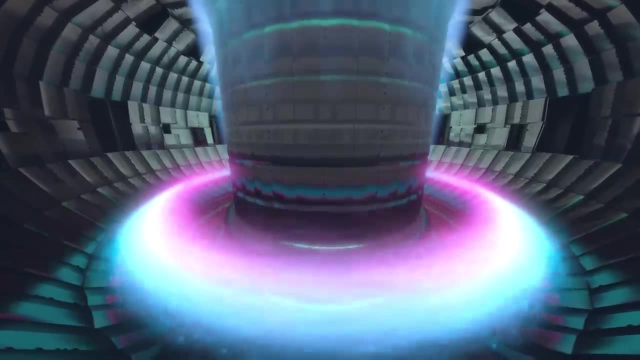 ITER will use three different heating methods to heat the plasma. The changing magnetic fields that will be used to contain the plasma create a high-intensity electrical current, creating resistance among the plasma. This is called ohmic heating and is the same method your toaster uses to heat its coils. 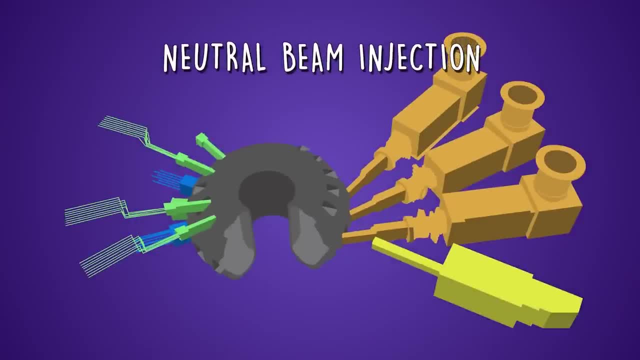 The second method is called neutral beam injection. It involves shooting high-energy particles into the plasma, similar to shooting steam from a cappuccino machine to heat the milk. And the third method is by high-energy electromagnetic waves. Just like your microwave transfers heat to your food, these extremely high-energy waves 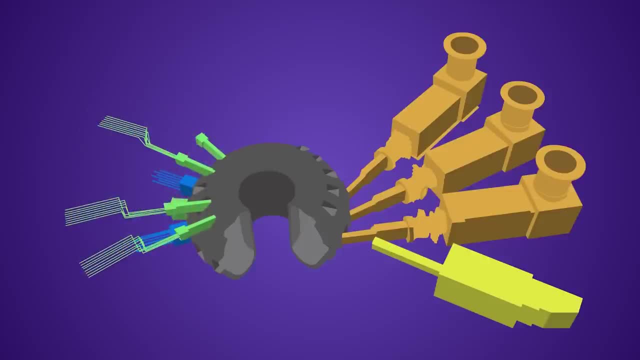 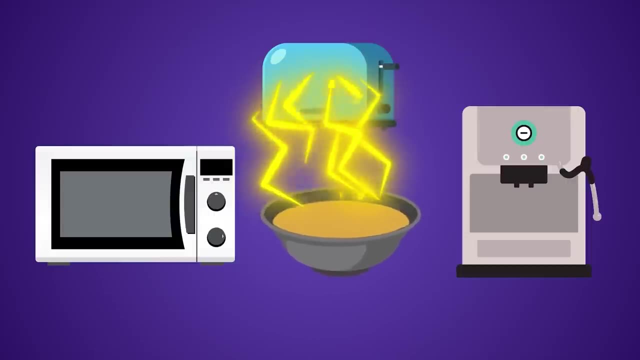 transfer heat to the plasma. You can think of it as three different appliances being used. You can think of it as three different things being used to heat soup all at once, Except the toaster generates a current of 15 million amps, about the same as 500 lightning. 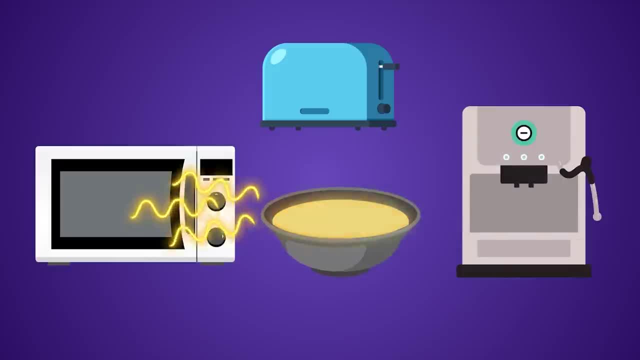 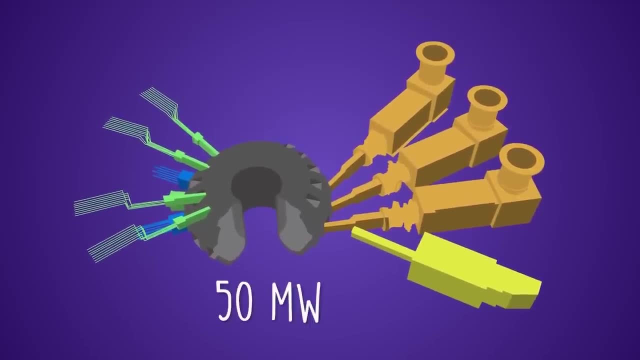 bolts, The cappuccino machine's power is closer to that of a jet engine, and the microwave can boost the soup to sun-like temperatures. Together, these three heating methods make up the 50 megawatts of input power. But how is that converted into 500 megawatts of fusion power? Nothing even close to this promised gain of 10 has ever been achieved, or even attempted to achieve. What makes the ITER tokamak different? The short answer is: the sheer size. The bigger the device, the higher the current and the more fusion reactions. 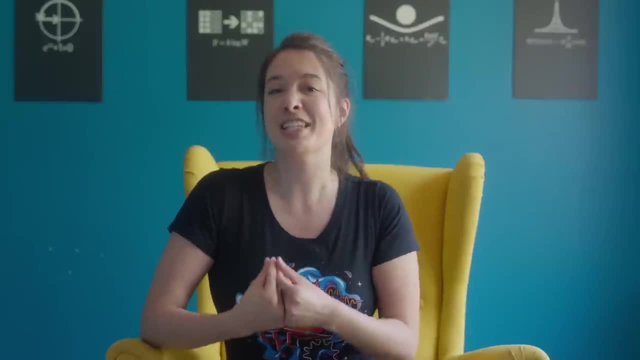 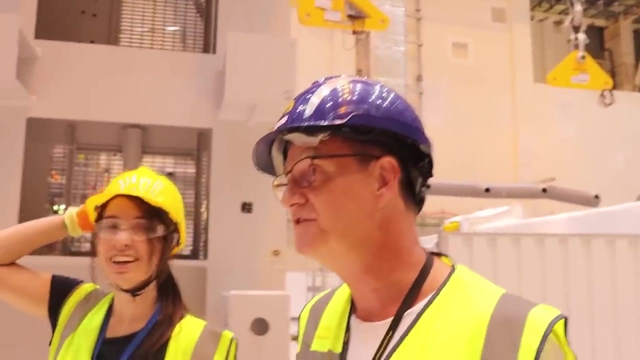 The long answer is so much cooler. As a physics grad, this was the highlight of the tour for me. This machine you're seeing here will be the first tokamak in which the dimensions are large enough for real self-heating to dominate. 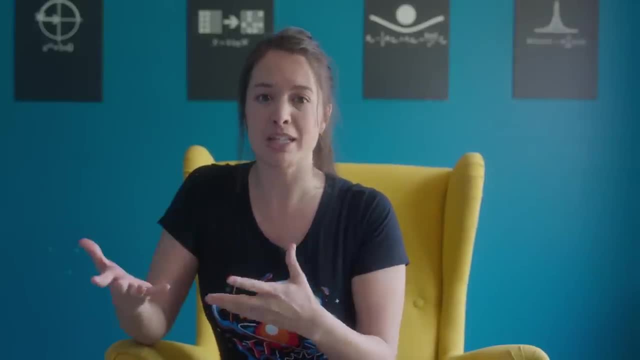 Did you hear that? Self-heating. Once we get the plasma to a certain temperature, it will be able to heat itself up. Once we get the plasma to a certain temperature, it will be able to heat itself up. Once we get the plasma to a certain temperature, it will be able to heat itself up. 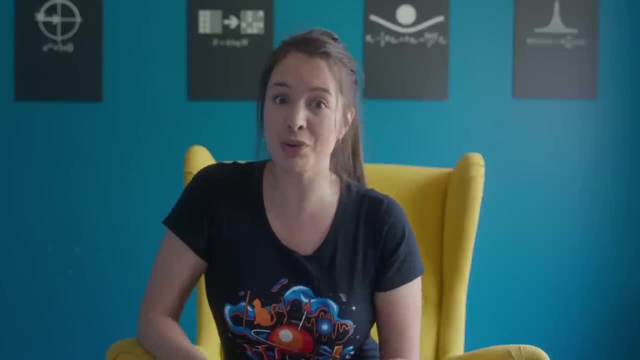 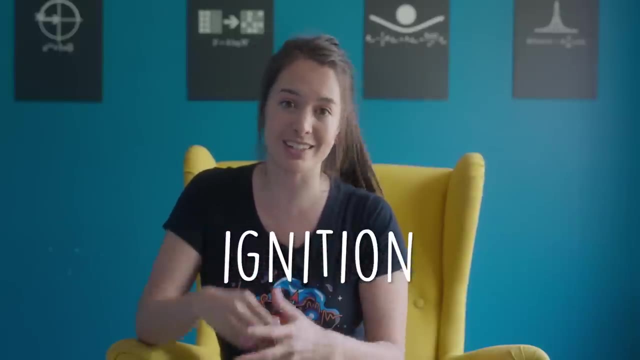 Once we get the plasma to a certain temperature, it will start heating itself, basically doing all the work for us. This is called ignition and is based on the same principle of why stars can burn for billions of years. So how does it work? 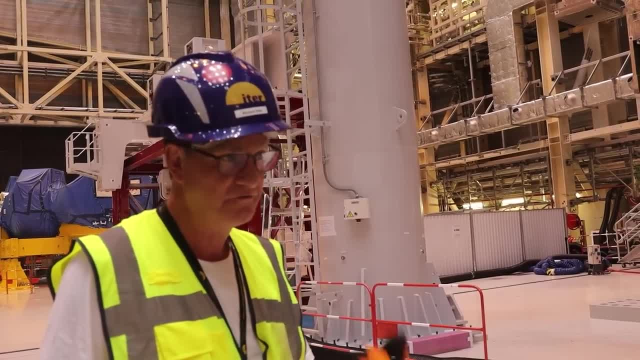 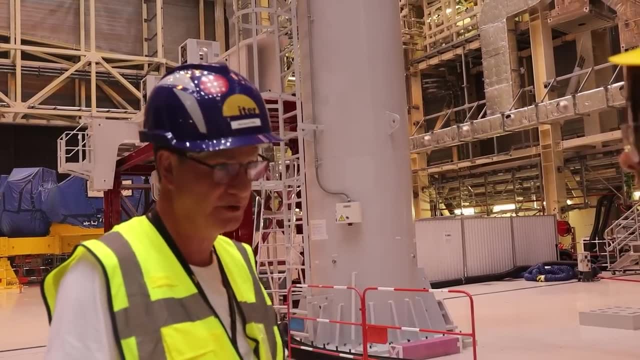 Of that power, four-fifths of it are in neutrons and one-fifth is in these helium nuclei that come from the fusion of deuterium plus tritium, And the helium is what's self-heating the plasma to keep it at burning temperatures. 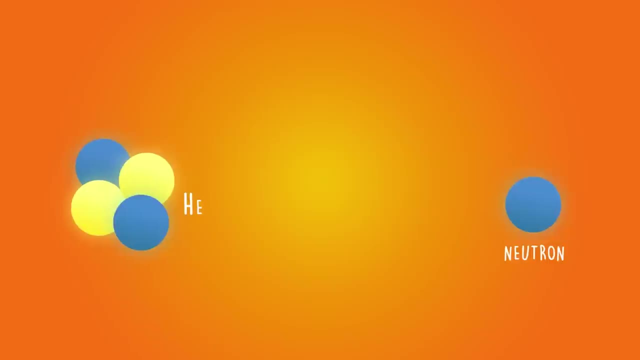 When the deuterium and tritium fuse, they release a neutron and a helium particle. We'll find out what happens to the neutron later. but the helium particle is the star of the show here. It's electrically charged, so it remains inside the magnetic fields with the rest of the plasma. 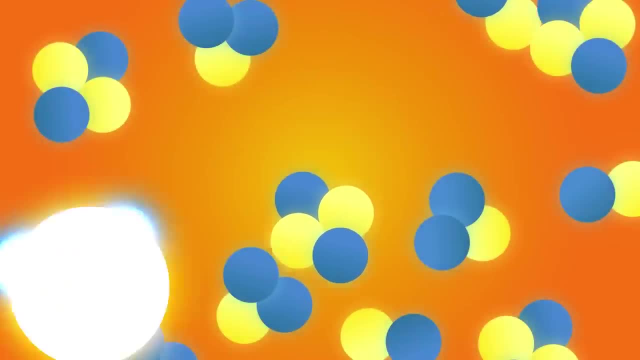 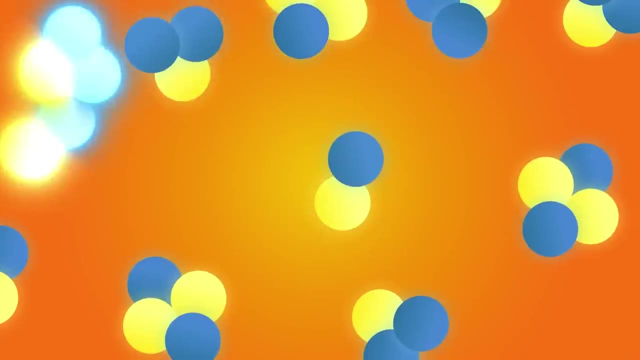 It's so energetic from the reaction that it whizzes around at lightning speeds, bumping into other particles, transferring its kinetic energy to them. The more energetic the plasma particles are, the more likely they are to fuse. Remember, heat is just particles in motion. 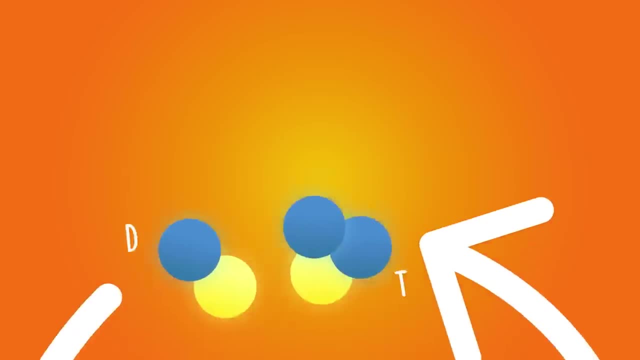 The faster the particles are moving, the hotter the plasma. So the fusion reaction produces a high-energy helium atom which transfers its energy to other particles in the plasma, which makes fusions more likely to occur. The more fusion reactions occur, the more helium atoms are produced. 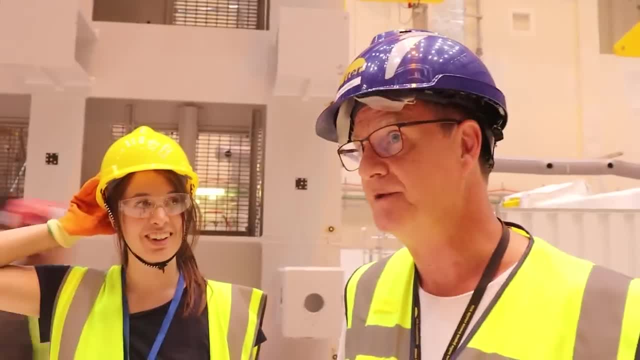 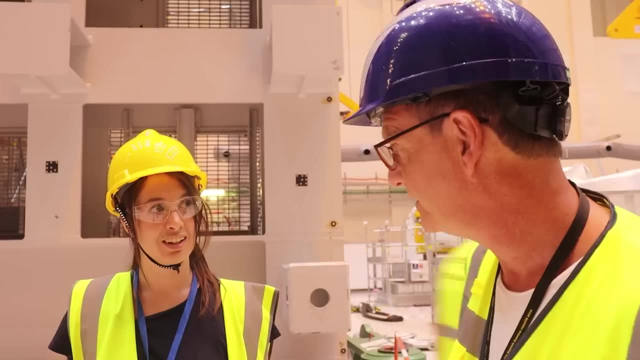 and on and on in an elegant cycle of self-heating The helium nuclei, which we call alpha particles. they will heat the plasma more than any system that we can use to heat additionally, And that's called a self-heated plasma. But here's a question for you. 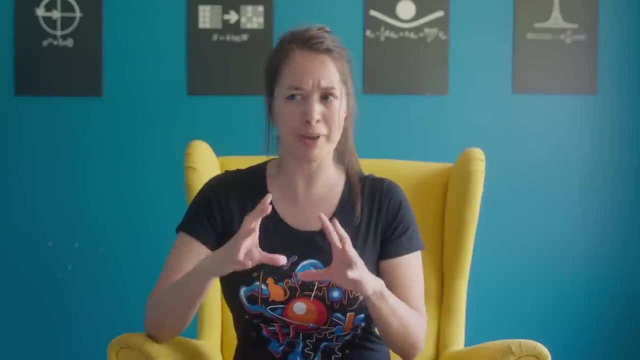 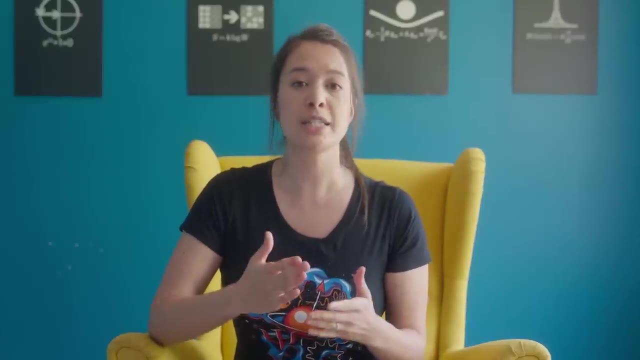 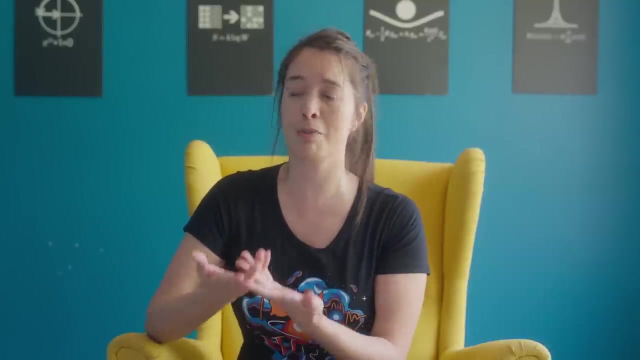 How is it possible to contain such large volumes of piping hot plasma? This is one of the biggest engineering challenges when it comes to commercial nuclear fusion. No material can withstand temperatures even close to 150 million degrees Celsius. I mean it's like trying to hold onto a piece of the sun. 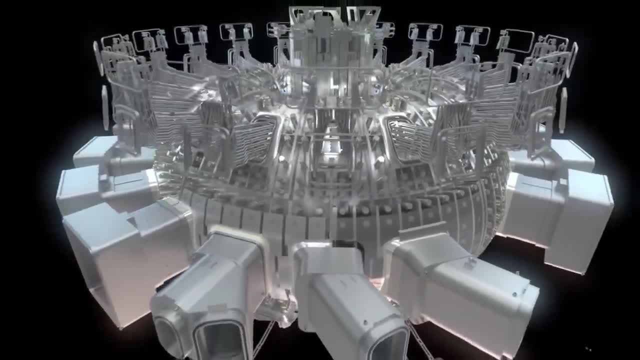 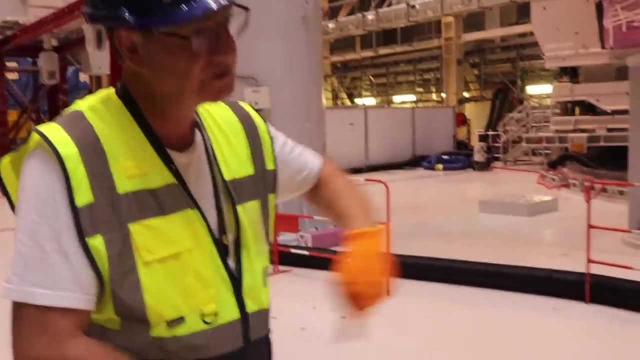 The answer is: what gives the tokamak its funny doughnut shape? The plasma stays confined because you drive a very strong, you establish a very strong magnetic field on the direction of the doughnut And the field is generated by these enormous magnets that you see. 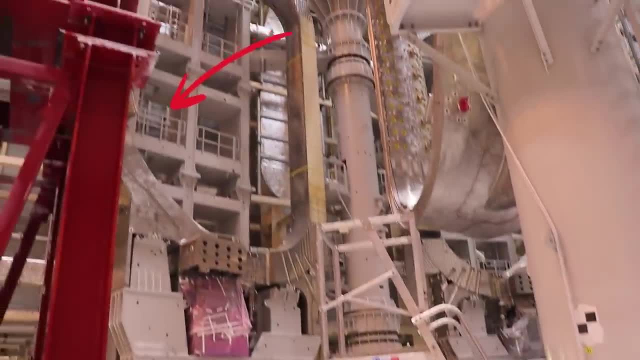 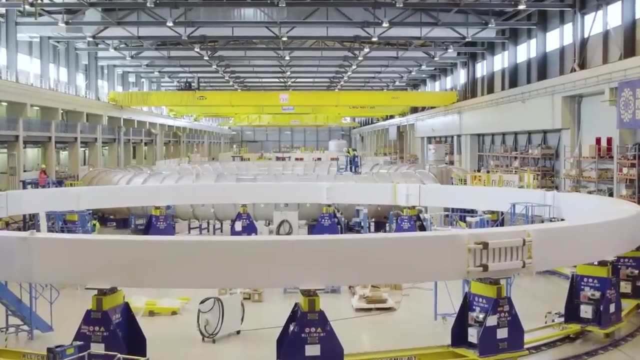 sitting on both sides of this particular sector. There'll be a total of 18 of these magnets in the ITER tokamak, each weighing 360 tonnes. When you combine these with the poloidal field magnets, that's 10,000 tonnes of magnets. 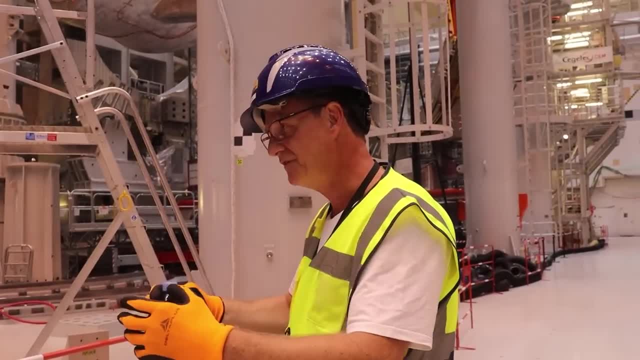 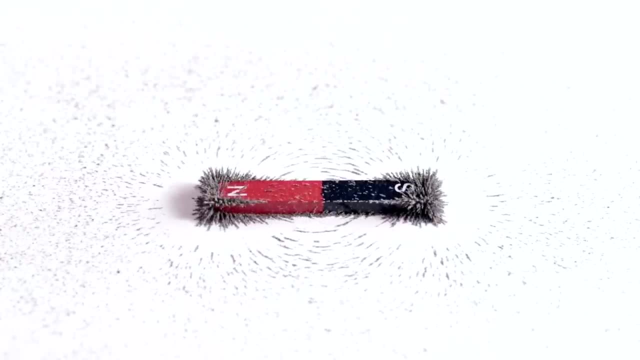 Why do you make the ring? Because if you want the plasma to stay confined, you want the magnetic field lines to close on themselves. Remember that plasma is electrically ionised, So, just like iron filings, plasma will follow these magnetic field lines. 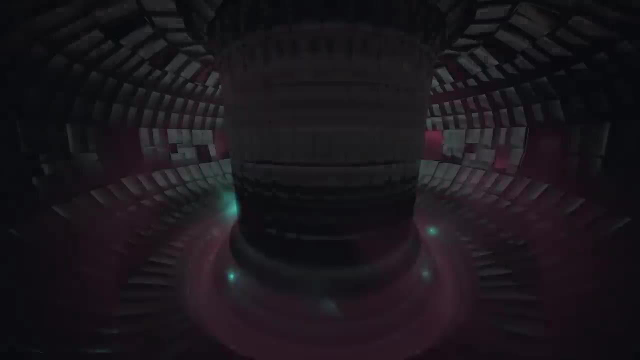 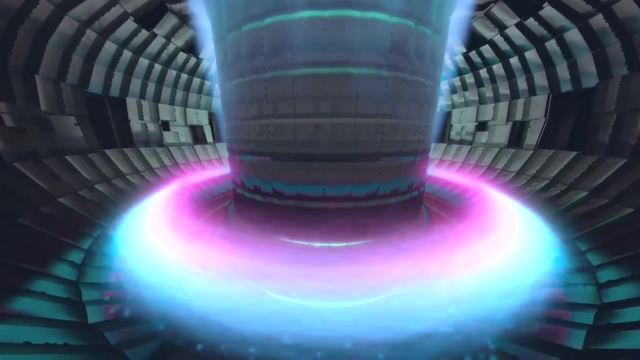 They're like invisible hands holding it in place. I think it's pretty cool how scientists exploited the electrical properties of plasma to contain it. It's like using its own power against it or something. If you want to make a fusion plasma from all the research we did in the last 70 years. 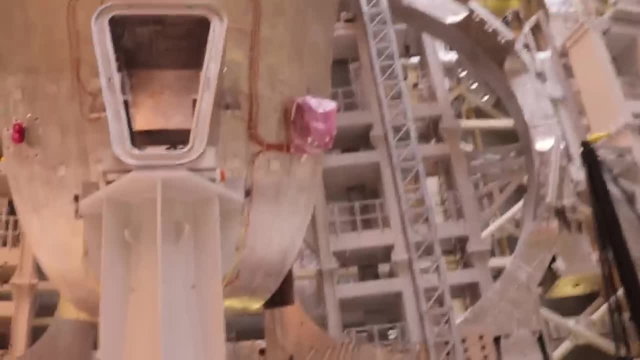 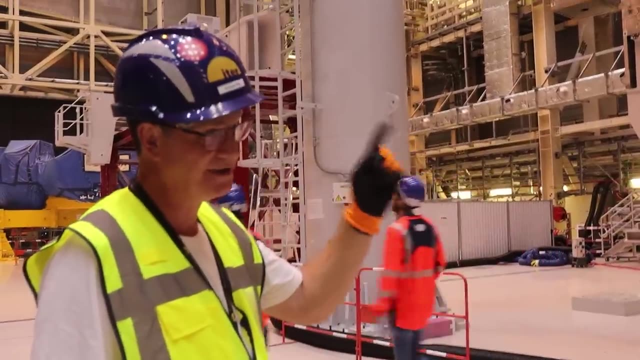 and you want to do it with a conventional tokamak design with fields, magnetic fields, which are possible on this scale using current superconducting technology. this is about as big as you can make it. These magnets produce fields of nearly 12 Tesla. 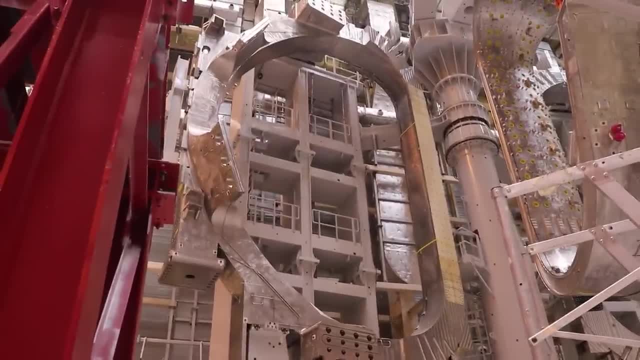 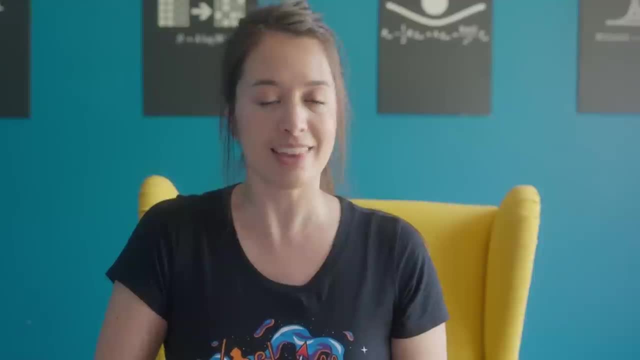 about 200,000 times stronger than Earth's magnetic fields. To achieve these crazy strengths, they need to be kept at 4 Kelvin or minus 296 degrees Celsius. That's colder than Pluto In a superconductor that you need for long-pulse tokamaks. you have to operate the coils in today's technology at a few Kelvin, so very close to absolute zero temperature. So you have a temperature gradient from degrees positive Celsius through to minus 269 in a few tens of centimeters, And you do that by making a thermal break. 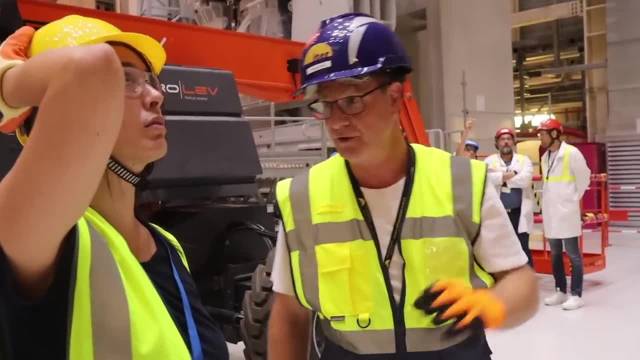 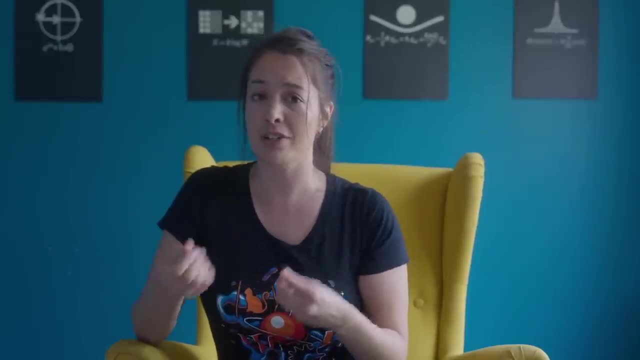 And that's why you have that 80 Kelvin shield in between, And that's the only way that this can be done. That's incredible. No doubt that this is fascinating and just really cool science, But how will any of this actually generate electricity in a real power plant? 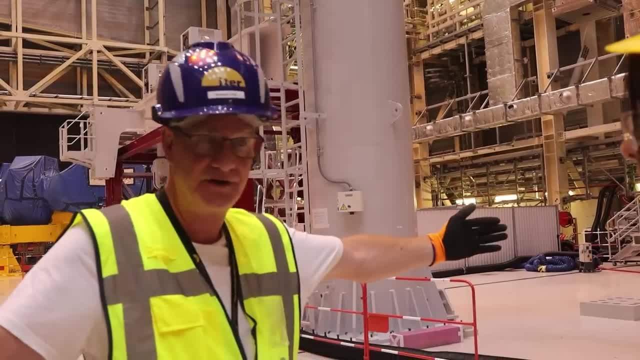 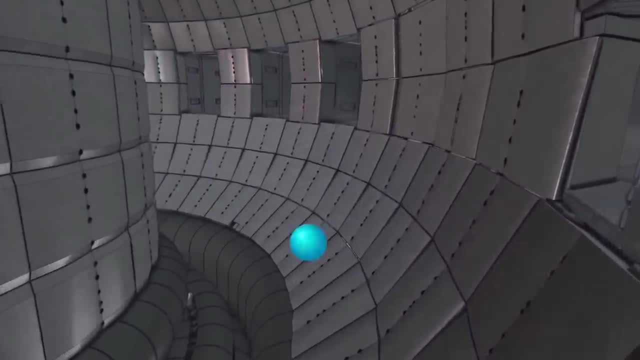 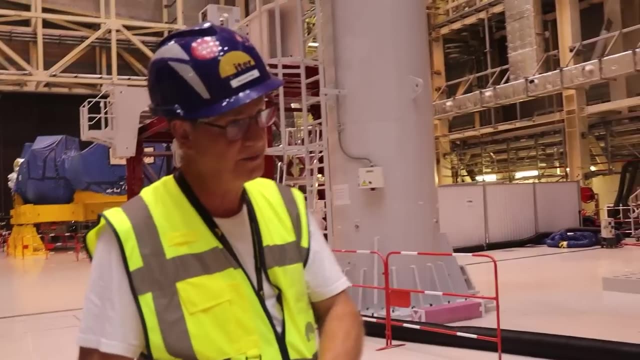 This is where the neutron shines. Neutrons just escape. They're not sensitive to the magnetic field. They are embedded in the wall, Not the walls of the vacuum vessel, but the blanket that we put in front of the vacuum. So this vacuum vessel will be clad with a huge first wall armor. 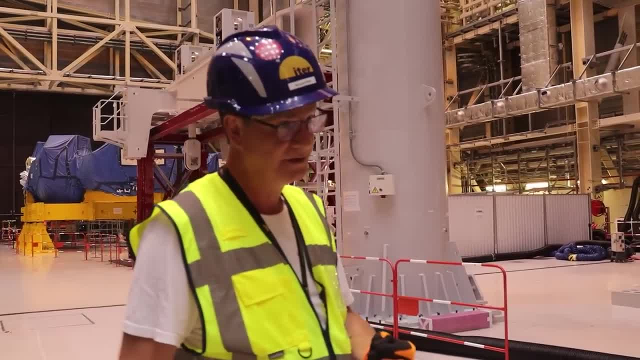 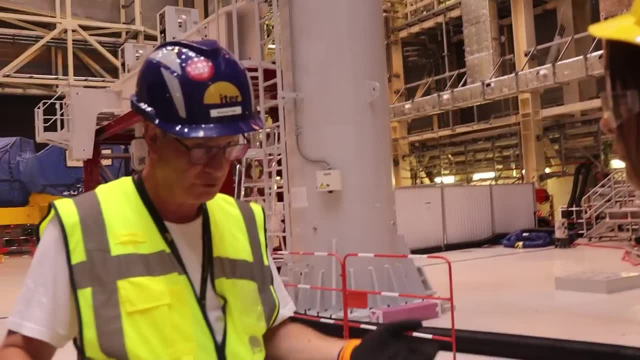 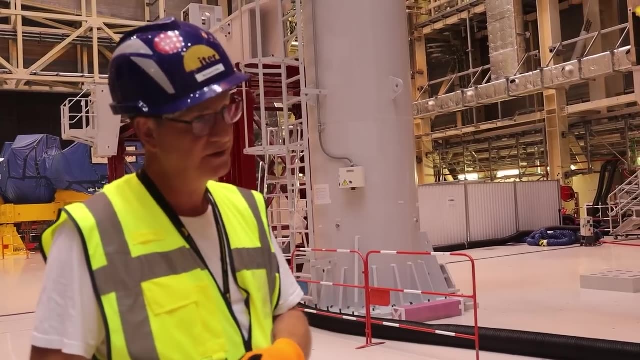 which is about 50 centimeters thick, made of steel, And that blanket will absorb the neutron power. In a reactor. the blanket will be full of cooling fluid and that fluid will heat up because the neutrons deposit in the blanket And then that will be used to drive turbines through heat. 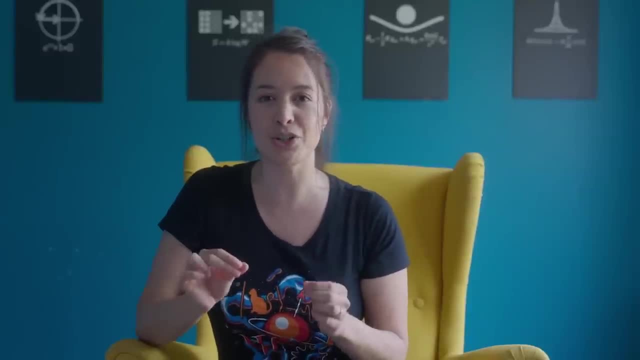 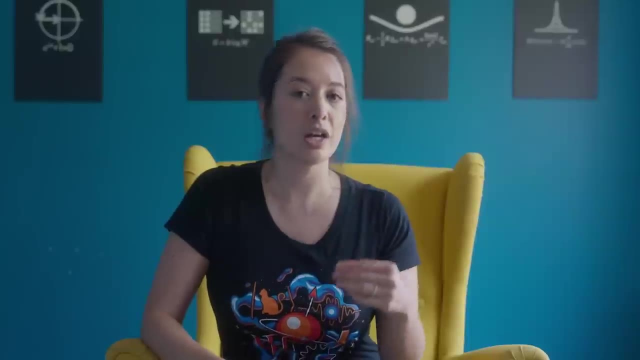 While the tokamak is the heart of the EDA project, the bones and sinews that hold it together, the civil engineering, the infrastructure, the vast support systems are equally fascinating When it comes to showcasing the sheer scale and engineering prowess behind this project. 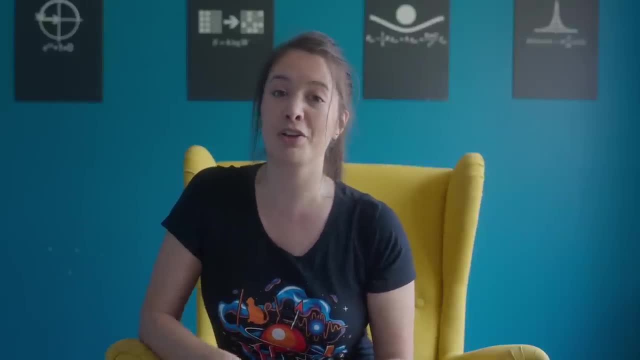 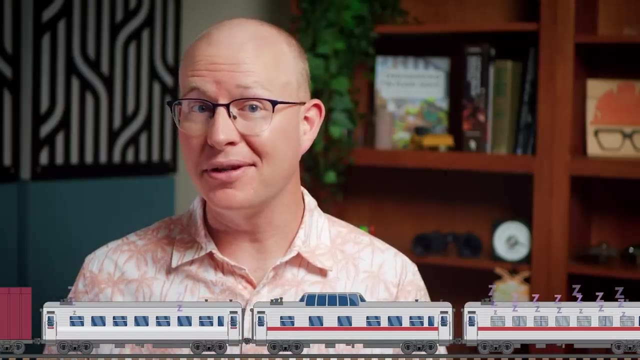 there's someone better suited to the job. I've asked my friend, Grady from Practical Engineering to share his experience with us. Grady makes wonderful videos about all things human made and he's been exploring the massive structures and systems that make ETA possible. 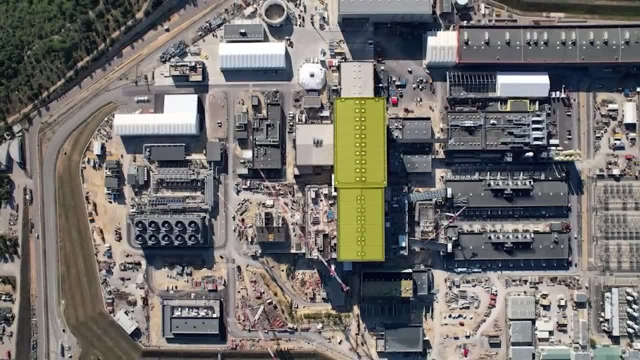 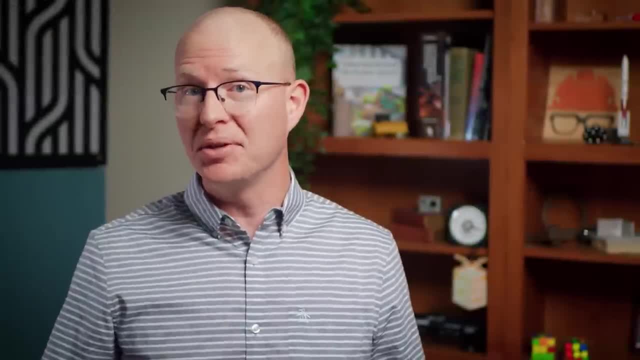 So far, we've really just been inside this building, Grady. what is all of this? One of the reasons ETA is such a grand project is that before they could start building the reactor, they had to build the buildings that would build the reactor. 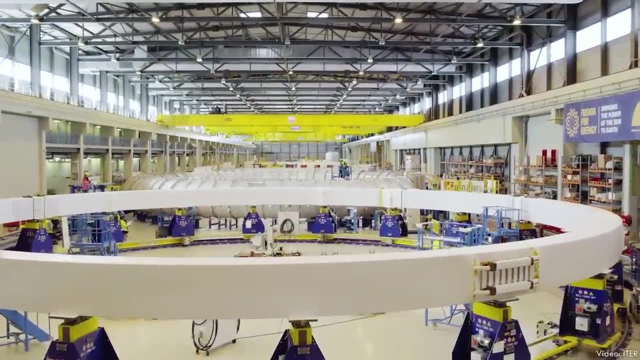 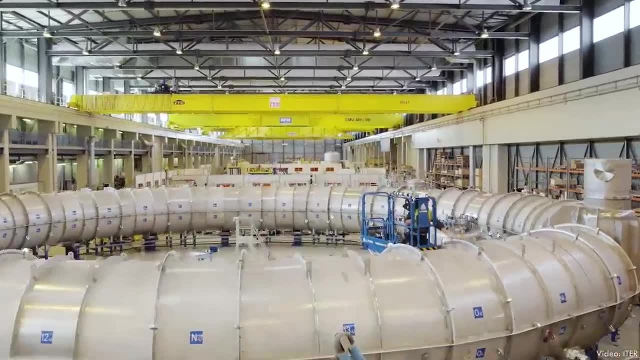 The magnets around the circumference of the tokamak, called paloidal field. coils are too big to transport on roads, so they're being constructed on-site in a dedicated manufacturing facility. Same thing with the cryostat, the enormous vacuum chamber that's. 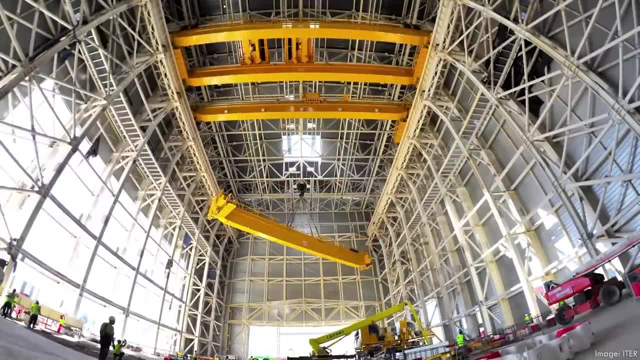 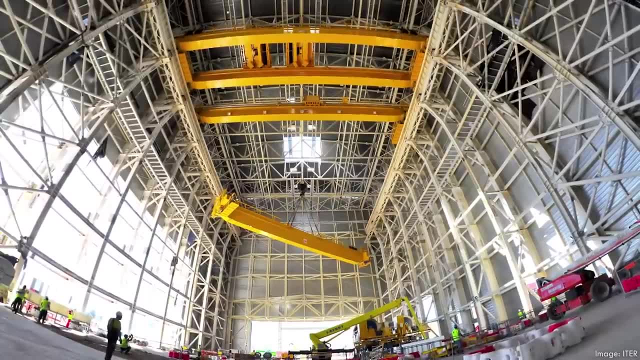 surrounded the reactor. Even a large part of the tokamak complex itself is a gigantic building with a set of gigantic overhead cranes dedicated just to getting the thing put together. But once the experiments get underway, there will be a lot more to ETA than the reactor itself. 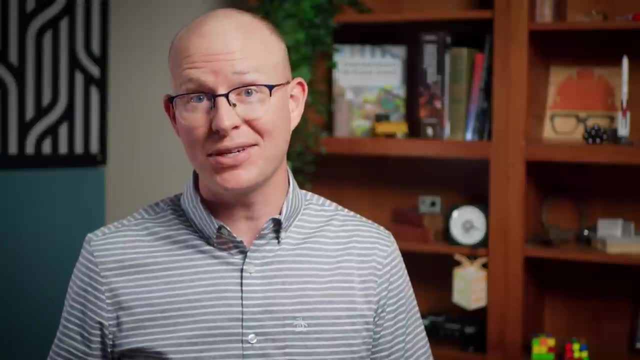 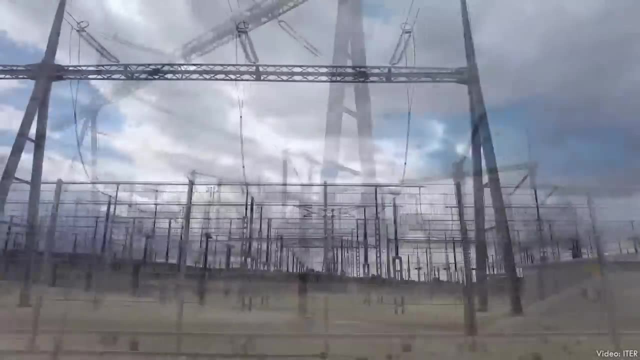 It takes power to make power, as they say, and that's especially true during plasma production shots in nuclear fusion research. All the electricity for the facility comes in through a 400 kilovolt transmission line, which is so high that it's impossible to get it to work. It's so. 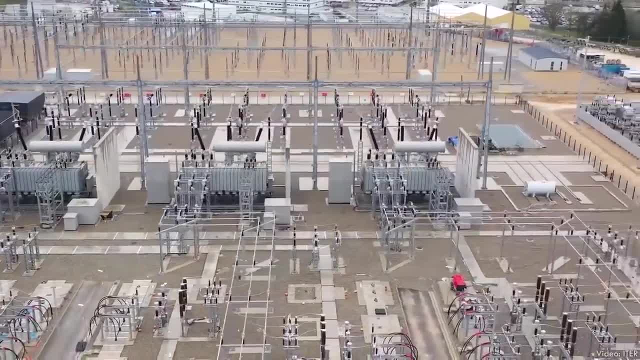 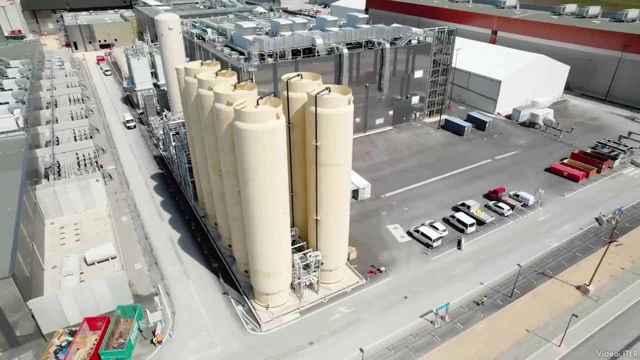 low that it's impossible to get it to work. It's so low that it's impossible to get it to work. Some of that power flows to the cryoplanet that chills and circulates liquid helium and nitrogen to keep the magnets cold enough to act as superconductors. Some of the power flows into 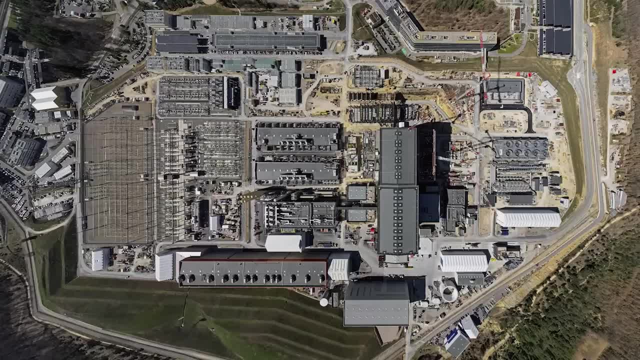 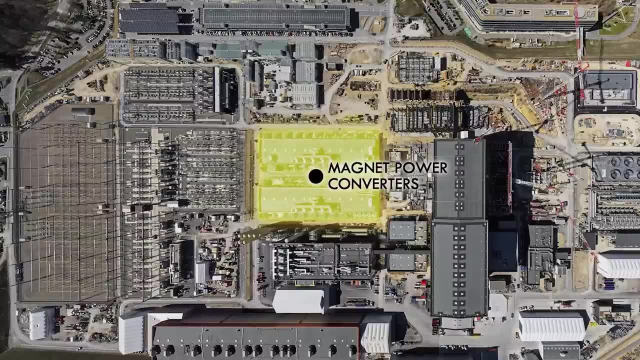 the magnet coils themselves. but before it gets there, it gets converted from alternating current to direct current in an industrial-scale power adapter that takes two buildings to fit. Finally, much of the power flows to the plasma heating systems that Jade already covered. Hopefully ETA will be able to do more than just that. We'll see. 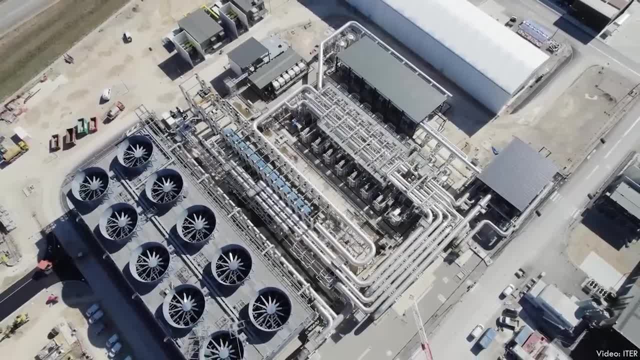 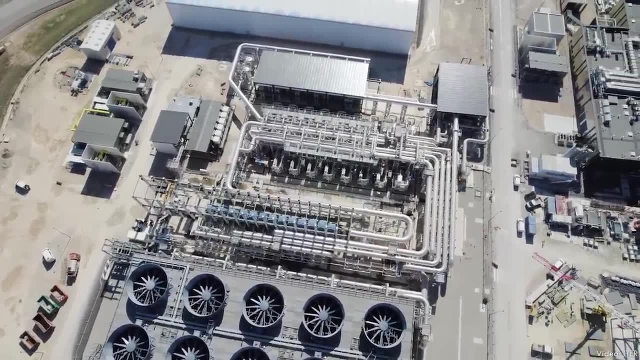 Hopefully that power is magnified during the experiments. but since ETA isn't converting the thermal output into electricity, it also has a water circulation system and enormous cooling tower to reject the output heat to the atmosphere. Containing a star on Earth takes some pretty 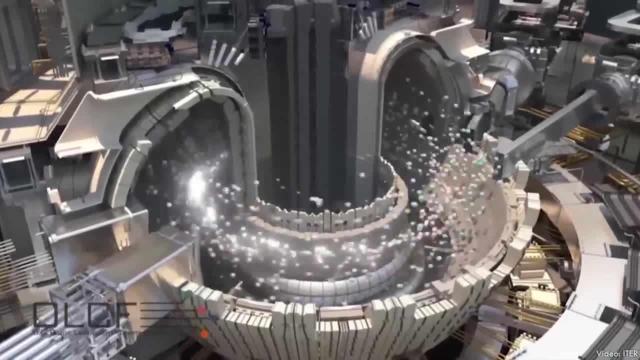 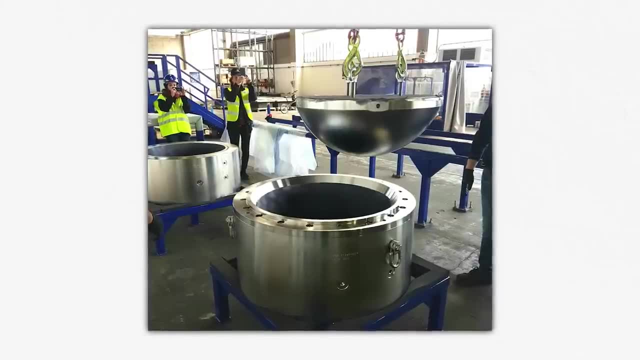 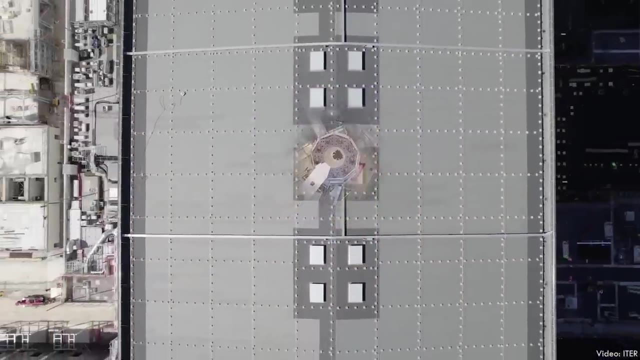 serious science. but just containing that container is a challenge, especially because it weighs 23,000 tons. The tokamak sits on huge spherical bearings that support the weight of the machine while still allowing it to shrink as it takes it. But even containing the container of the container requires a special consideration. 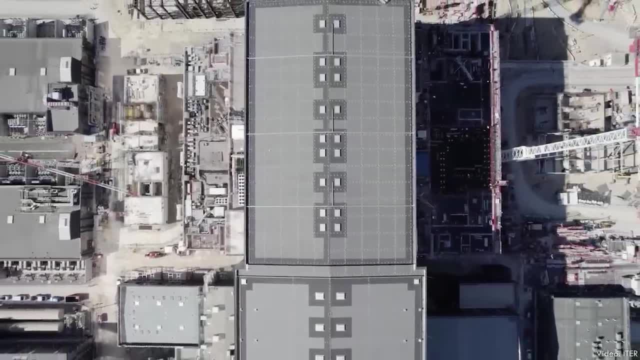 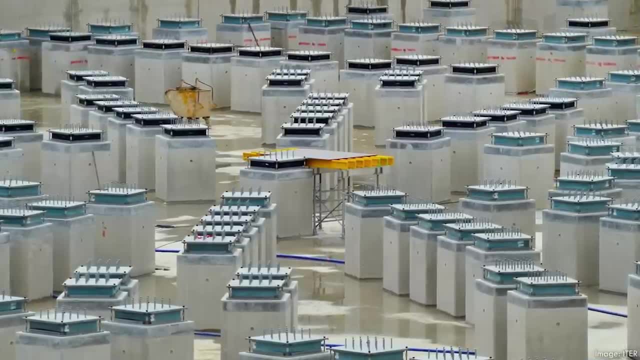 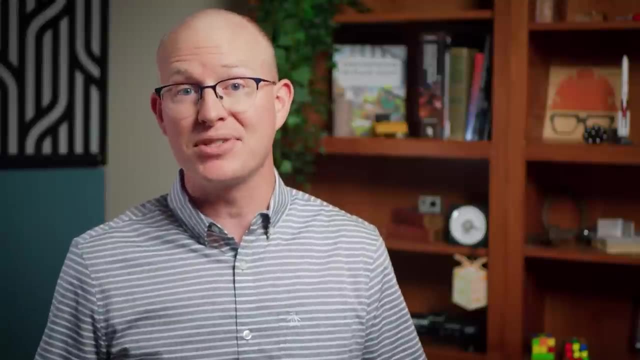 of disasters and threats like floods, airplane crashes and earthquakes. The whole building sits on a forest of concrete columns with bearings that allow it to move independently from the underlying soil, decoupling the building from any shaking that might threaten its safety. And that's just a few examples. 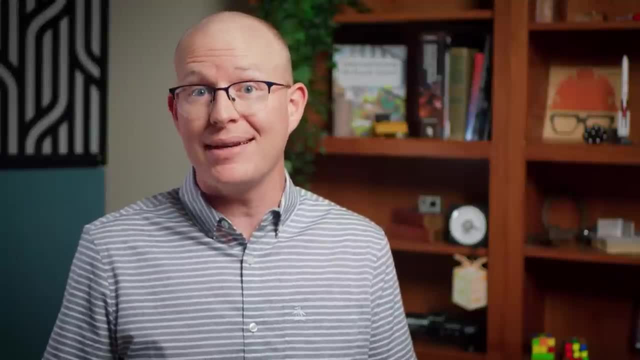 of the engineering at ITER being executed on a scale that's literally never been done before. But more importantly, it's not just the engineering at ITER, it's the engineering at ETA. For more of the construction side of ITER, make sure to check out Grady's video after this one. Which brings us to a question I'm sure a lot of you are wondering: When will construction be complete? When can we expect first plasma Back? when ITER formally began in 2006,, it was projected to take 10 years to build. Obviously, that deadline has been pushed back, with the ITER website saying that today they're. 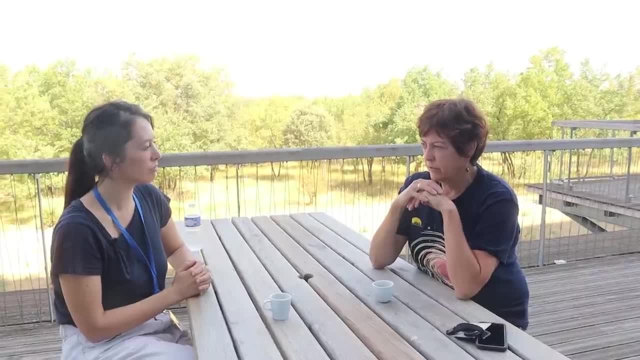 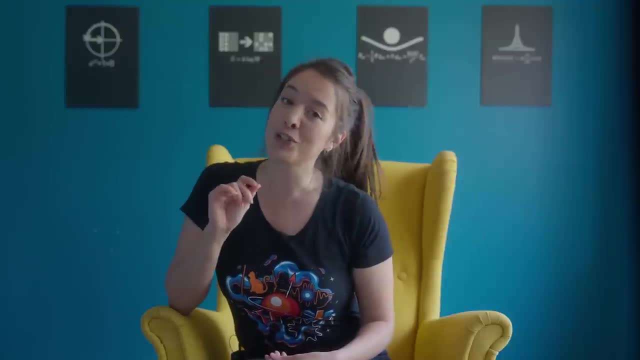 89% finished with construction. The date for first plasma was 2025. But this is not going to happen. I cannot give you a date right now. It reminds me of the old joke that commercial fusion is always 30 years away. 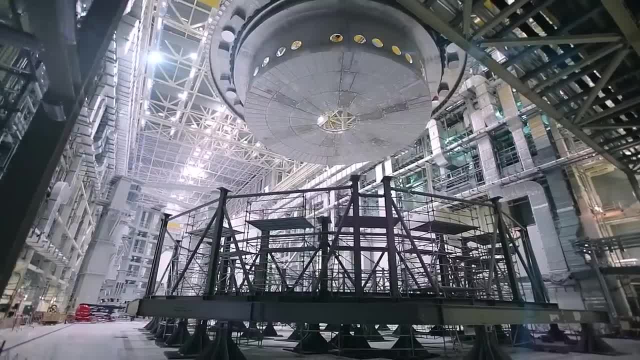 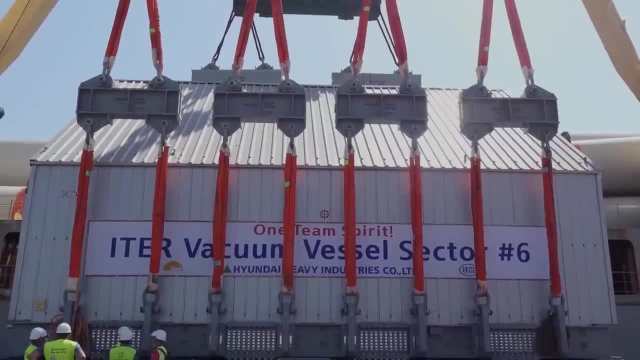 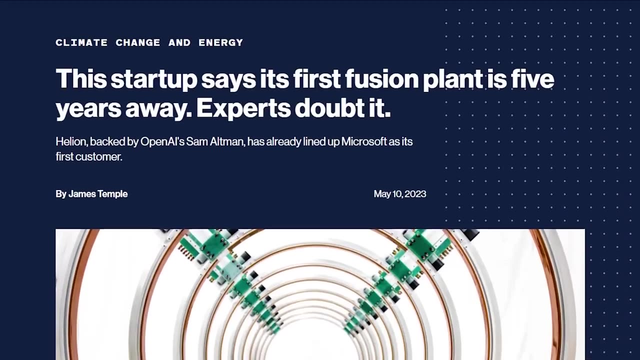 But is that still true in 2023?? The fusion landscape has undeniably transformed in the last few years. More money and resources are being spent on fusion than any other time in history. I keep seeing headlines about breakthroughs. Some private companies are even claiming to unlock fusion's potential within the next five years. 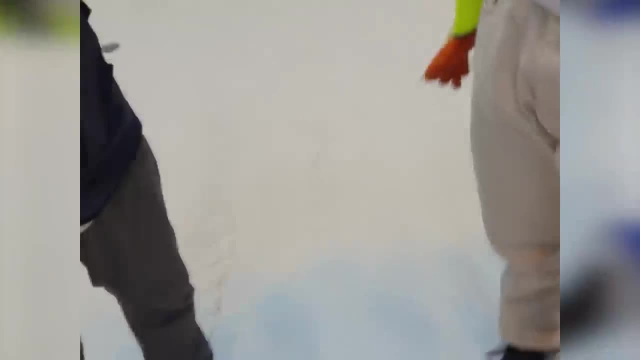 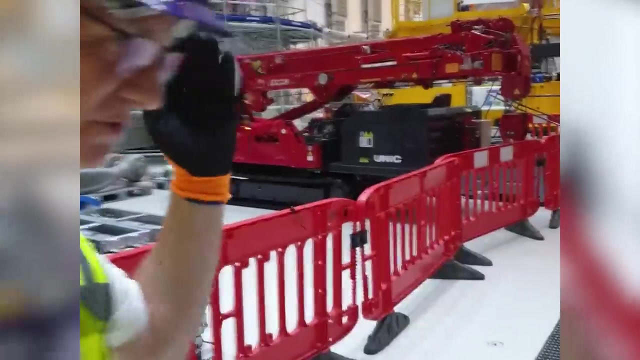 But not everyone shares this story, This optimistic outlook. I try to get this through to everybody who comes. There's a lot of hype. Again, these companies are using this. They're saying this: we will solve the fusion problem, We'll solve the climate problem. 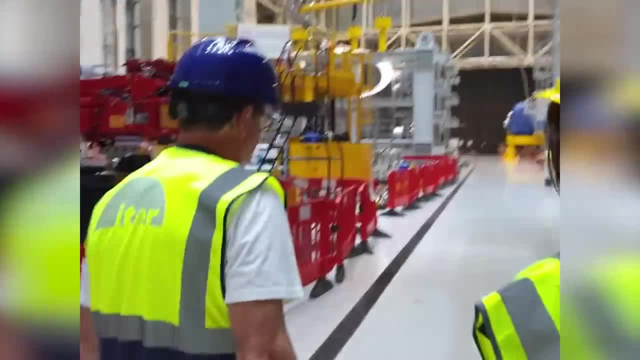 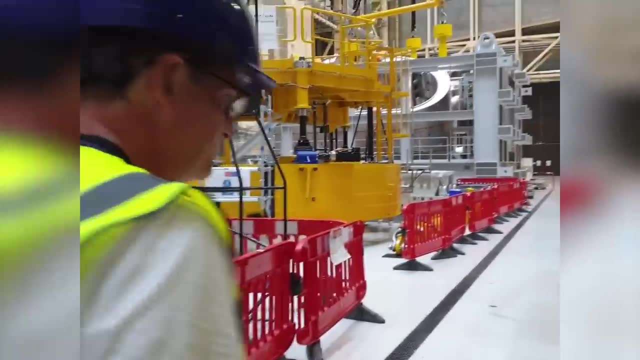 And they get money from people who can't stand it, because it's just not true. This reactor is 20 years away from burning, probably, And even when it's burned, and we've spent 10 years, 15 years operating it and learned. 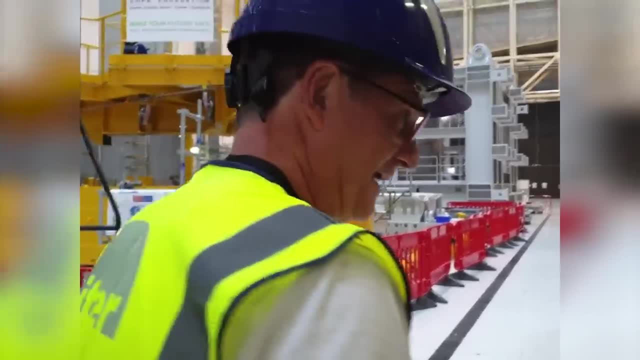 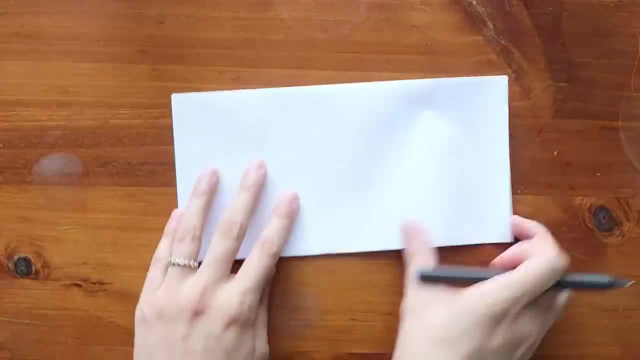 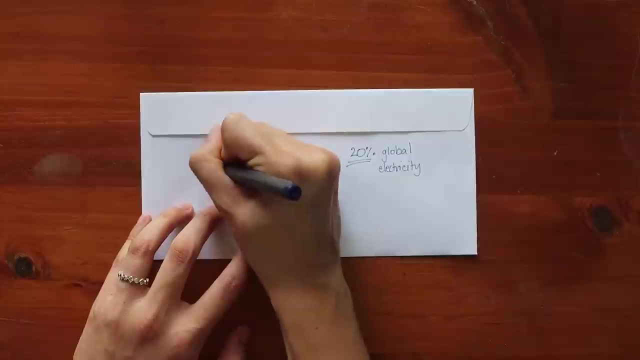 how to do it. you've got to build the demos that are real reactors that will run not for 2,000 seconds but 24-7.. Do a simple calculation: If you want to supply 20% of the world's electricity demand- 20% only by fusion- by 2080,. 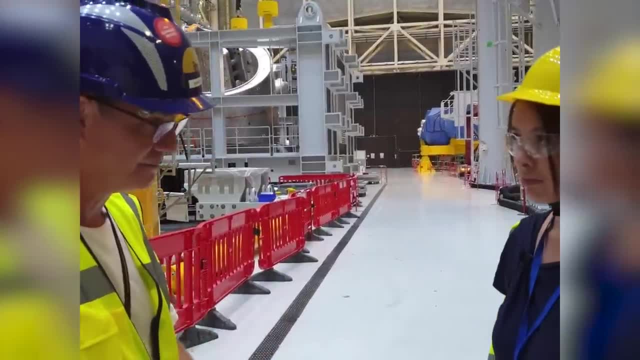 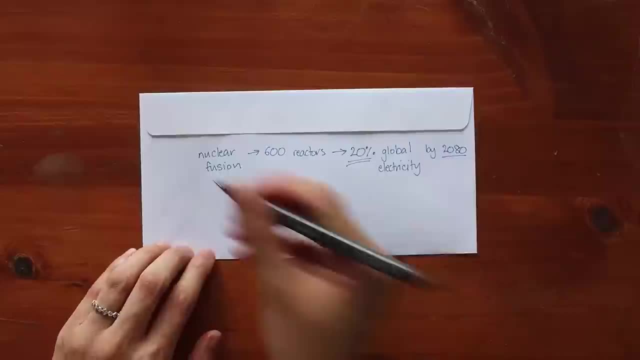 assuming we could build these things on a commercial scale by 2080 and have them all operating. you need 600 of them worldwide to produce 20%. Now look at today's nuclear fission: It's about 480 fission reactors. More or less Always working worldwide in all the different countries. It's producing 11% of today's global electricity demand, So my 600 is not far off Now. my reactors that I use to calculate that number were 2,000 megawatt electric devices. 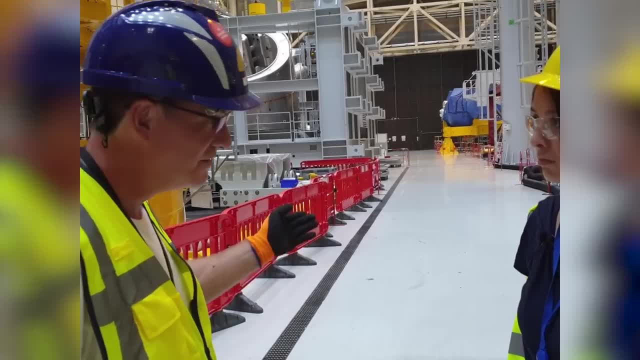 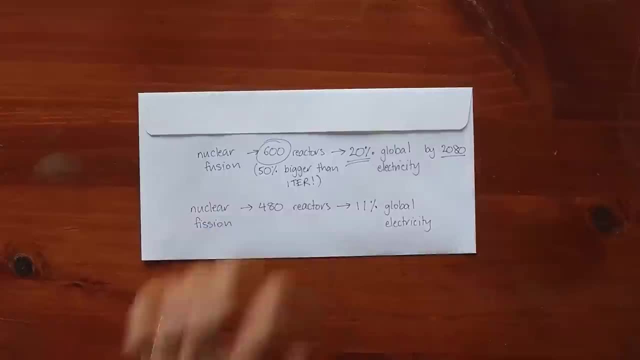 massively bigger than this, And we haven't even done this one yet. Bigger than this one? Yeah, Okay, You need to be 50% bigger than this to get to the 2,000 megawatt electrical scale, unless this new. 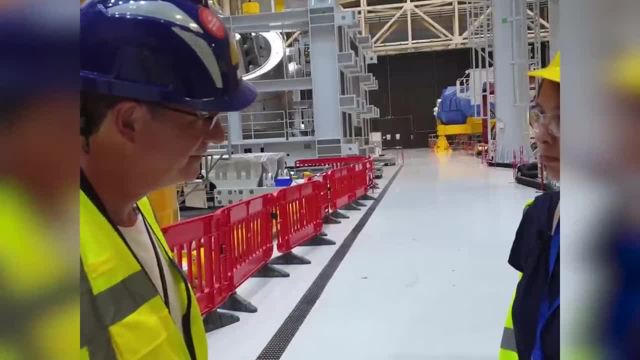 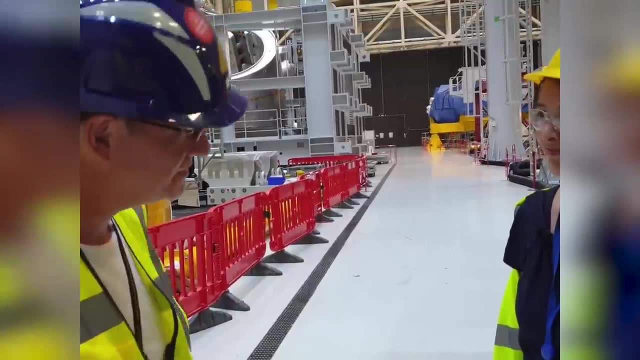 HTS technology works, But they are decades behind us, So I don't even think we can build a few of these by 2080, never mind 600. And then we're still only at 20%. Richard seemed to think that if we wanted commercial fusion by 2080,. 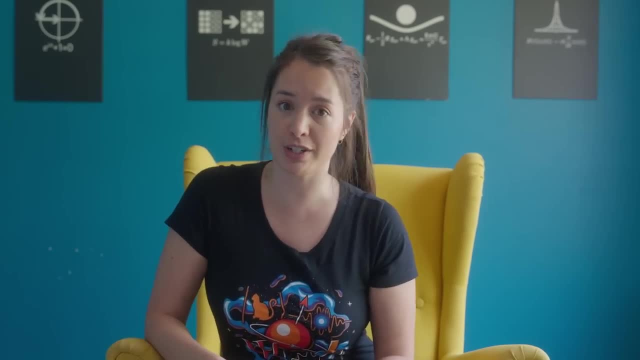 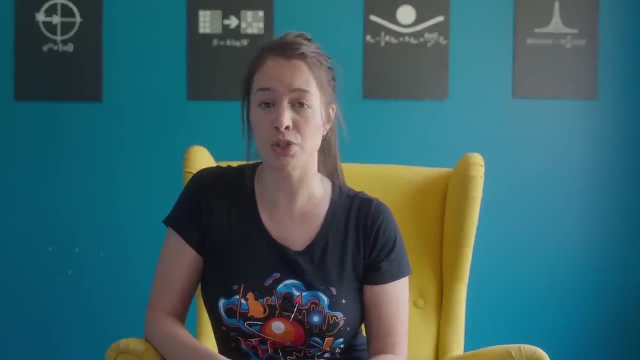 we'd need to do some kind of Manhattan project, but for nuclear fusion. You may have seen Oppenheimer recently. Very good film, Very good. I thought it was excellent That we won't reach commercial nuclear fusion in time to solve today's problems unless we 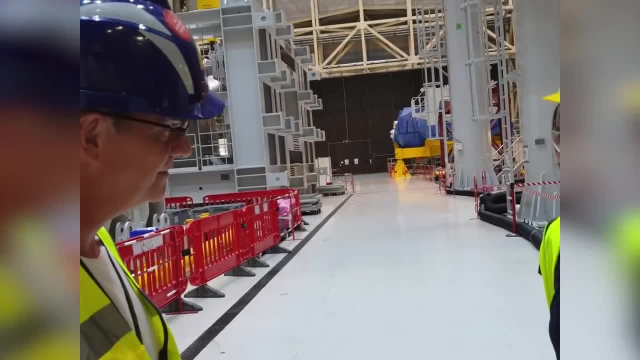 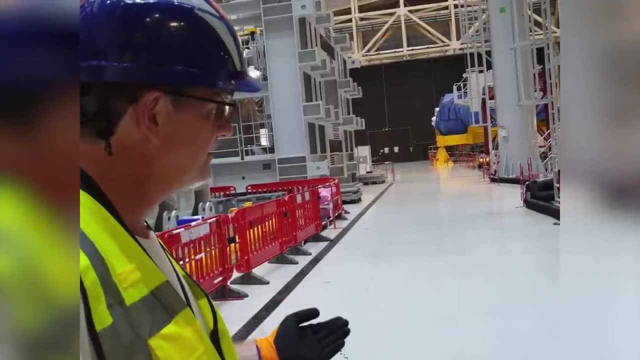 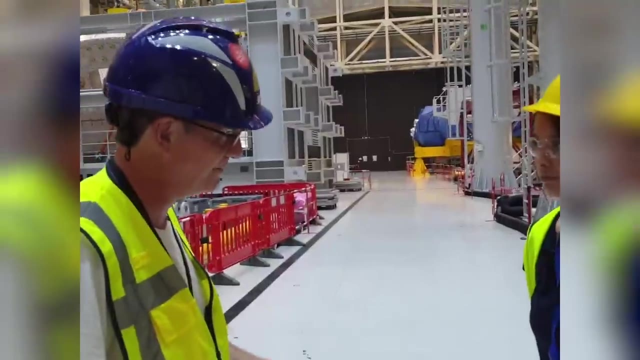 massively increase budget and effort. This is not the answer that we're doing. It's the answer for the longer term, because, even if renewables start to improve and get better and better and better, you still need baseload electricity supply, Something that's always there when the sun isn't shining and the waves are not waving. 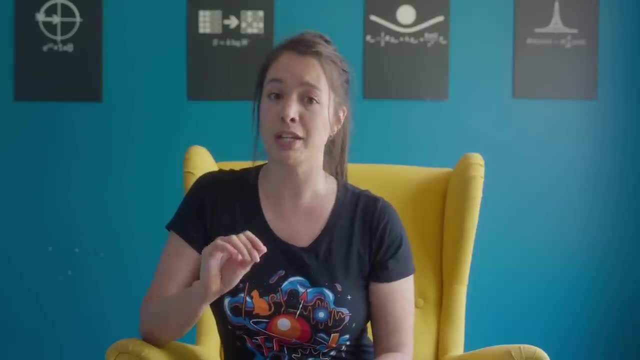 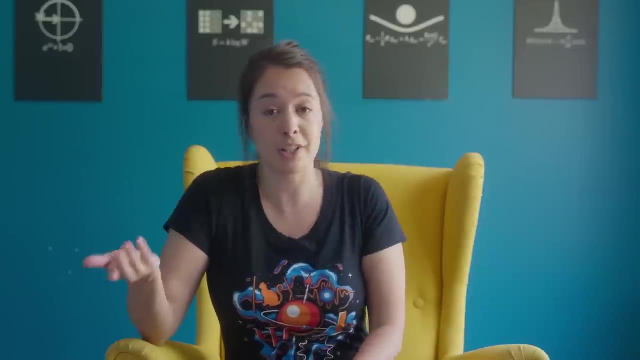 and the wind is not blowing. It's important to remember that Richard's opinions don't reflect those of ITER as a whole, But this is the first time I've heard a broken down argument of the timeline to commercial nuclear fusion, So that was really refreshing to hear. 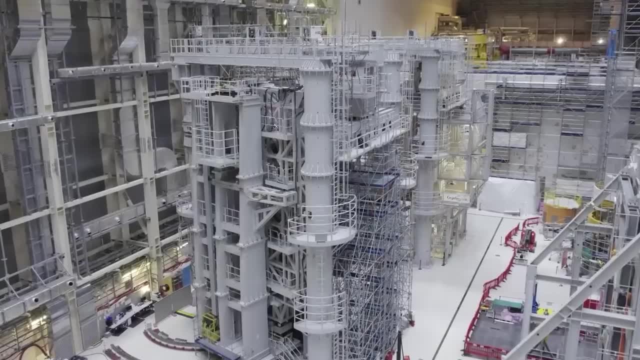 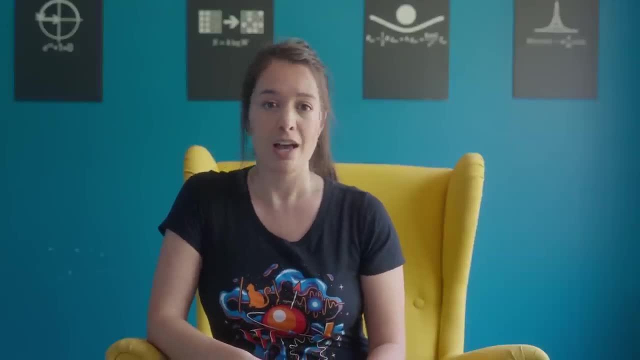 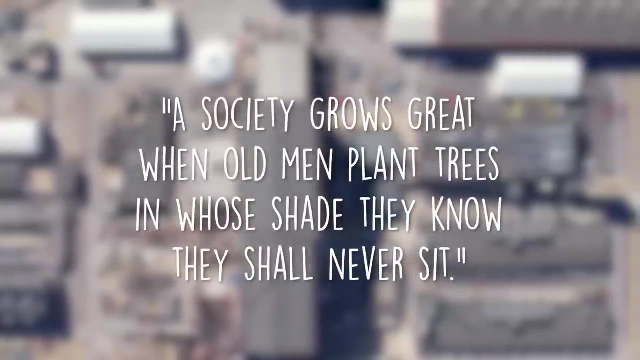 As technology advances and collaboration increases, there's always potential for timelines to accelerate. But even if Richard is right and we won't see commercial fusion until next century, I don't think that should dampen our enthusiasm. As the old proverb goes, a society grows great when old men plant trees in whose shade they 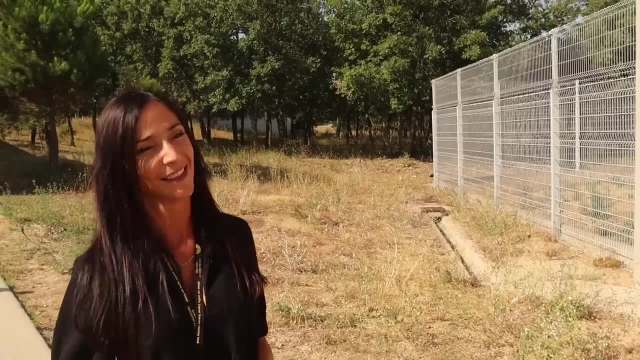 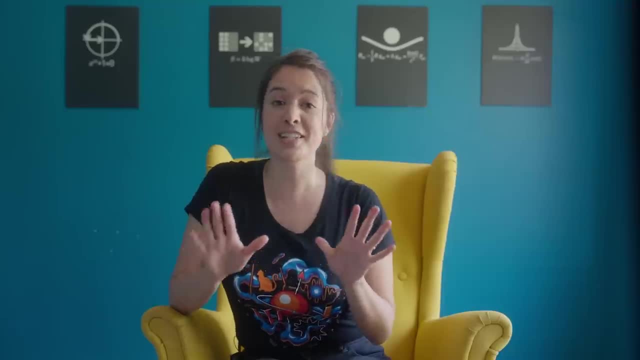 know they shall never sit. It's corny, but it's true. People who spend their entire life working towards a brighter future they'll never see are the people who change it for the better. Okay, so here's kind of a weird question. 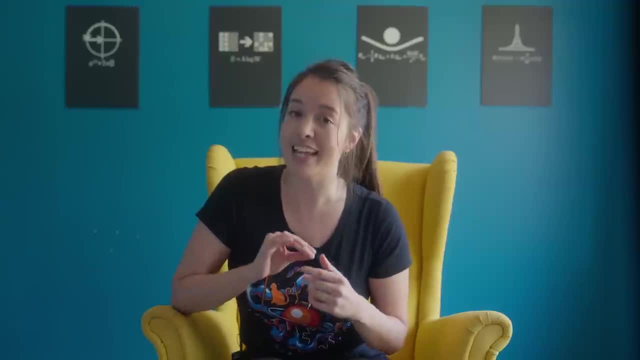 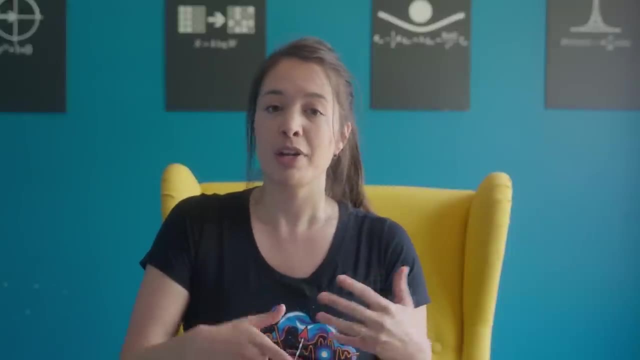 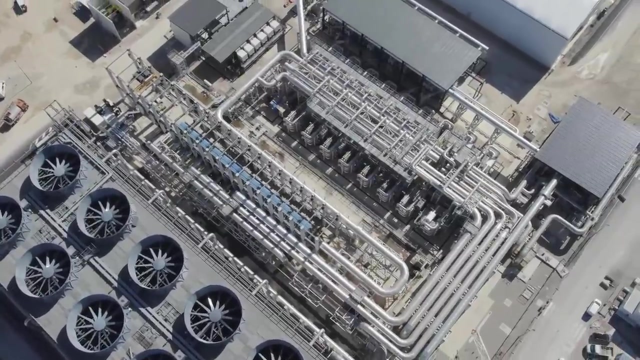 But do you think that if we ever met an advanced alien civilisation, that they would have a nuclear fusion plant like ITER? Here's why I'm not so sure They would have had to come up with the same mathematics as we did. Remember that none of this impressive engineering would have been possible without the mathematics. 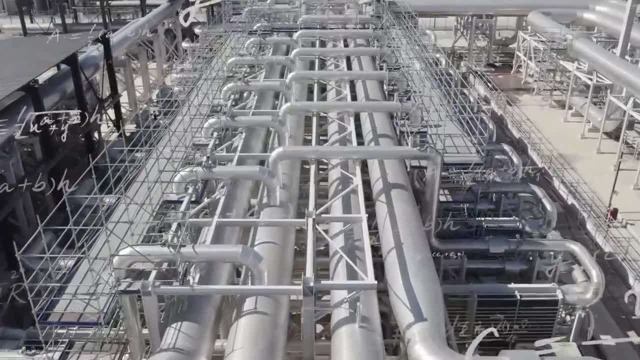 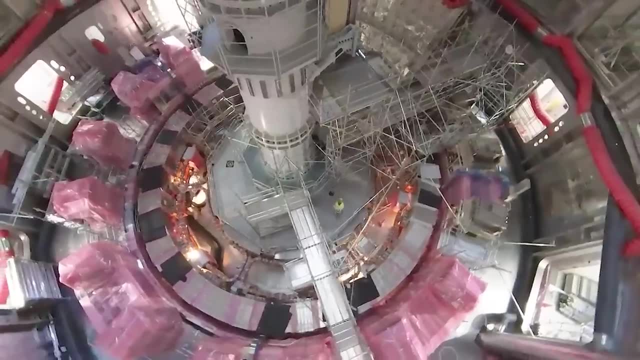 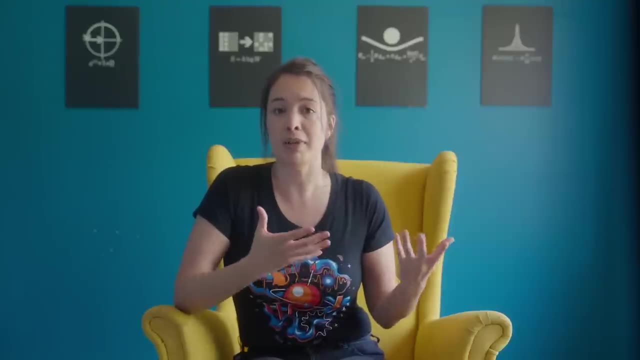 behind it And that mathematics took us centuries to develop. Every pulse reaction, every magnetic field line of ITER is described by an equation. There's no doubt that we invented this, But did we invent the math that makes them work? If math is a human-made invention, then it's not that likely that an alien civilisation 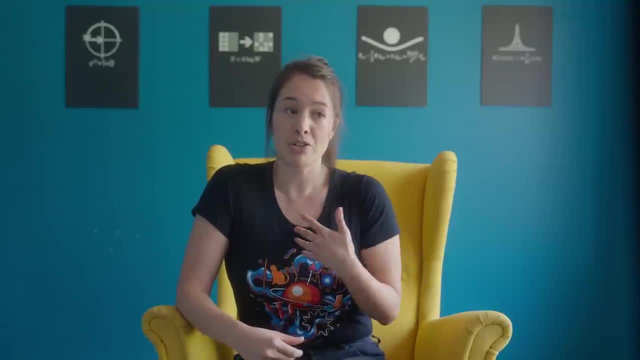 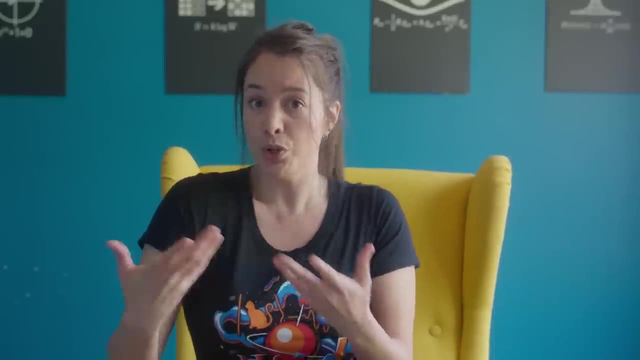 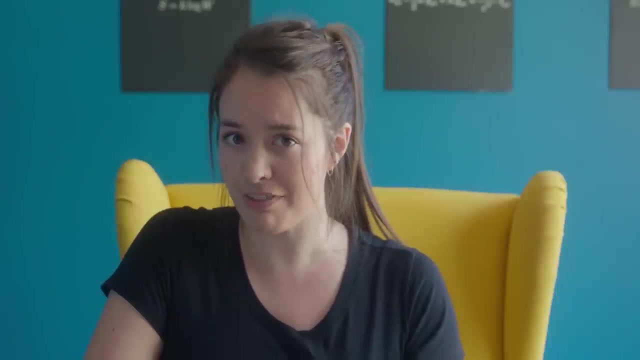 would have a similar nuclear fusion plant. Our inventions depend on the way we think. However, if mathematics was already there and we just discovered it, an alien civilisation would probably have discovered it too, right? This really boils down to the question: is math invented or discovered? 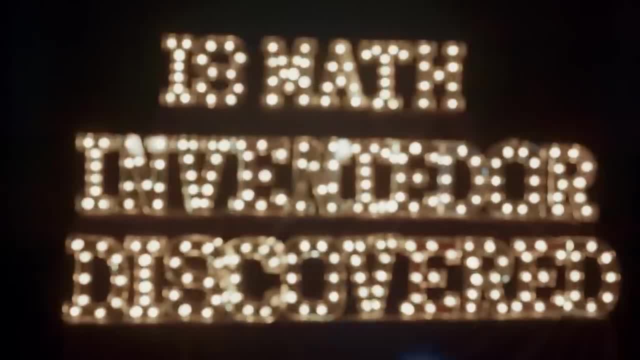 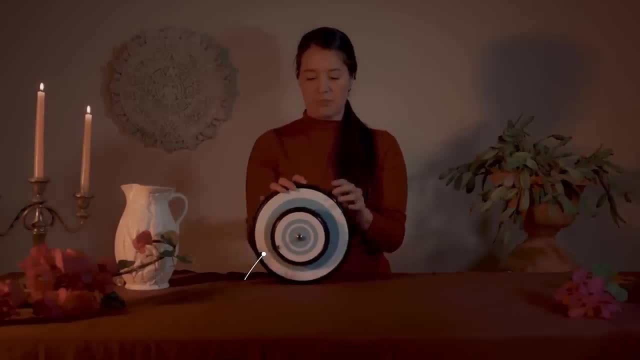 This question bugged me so much I made a feature documentary about it on Nebula. What's Nebula? Some creative friends and I teamed up with our own streaming platform where we don't have to worry about the pressure of the YouTube algorithm or clickbait titles to keep creating. 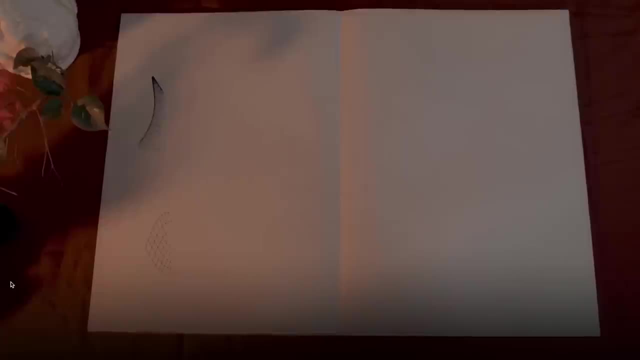 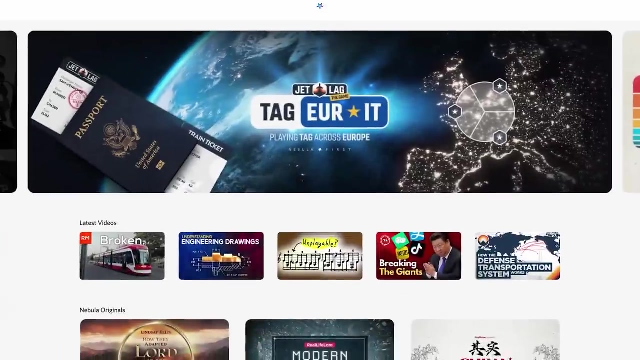 Nebula is a place where we can focus on passion projects, experiment with original content, all while staying completely ad-free. Nebula features a lot of YouTube's top educational creators, like Real Engineering, Joe, Scott, Wendover Productions, Tibbies and many more. 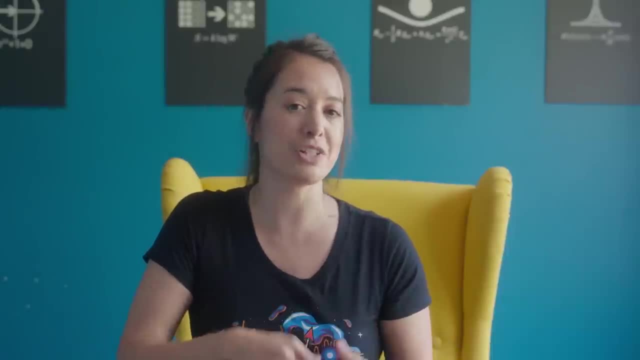 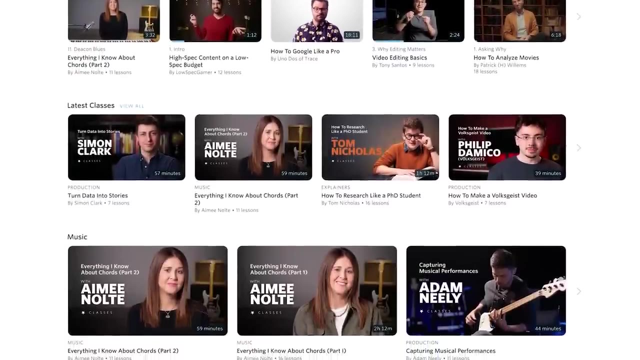 If you're a deep thinker and like to contemplate the boundary between math and philosophy, I think you'll like my documentary. They also offer classes led by creators teaching well how to create. Have you ever thought about creating your own science videos? 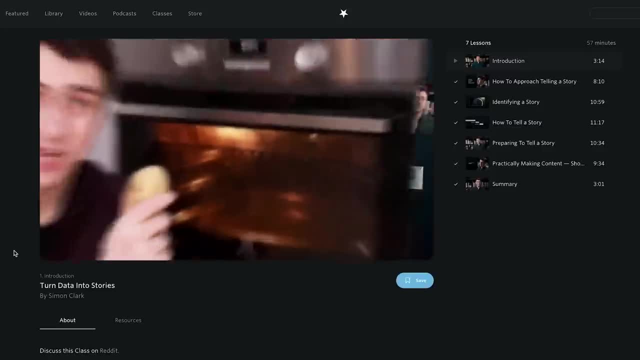 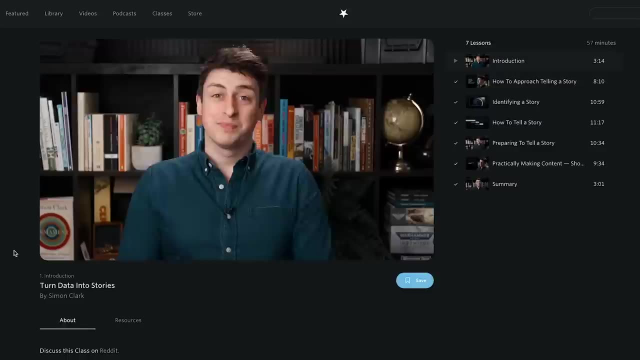 Or would like to level up at science communication in general, Then this class is for you. Turn Data Into Stories is a class taught by science YouTuber and climate science PhD Simon Clarke. He addresses questions like: how do I pick a story out of the data? 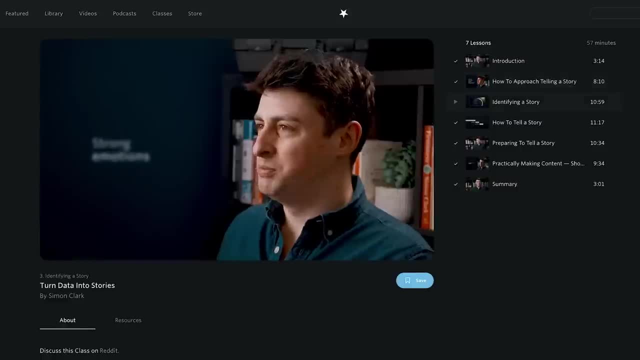 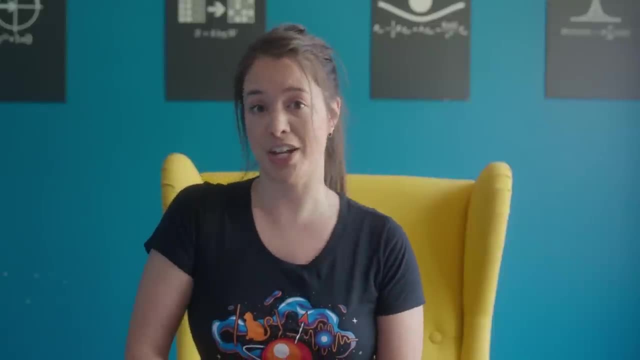 How do I decide the best way to visualise and communicate it, How do I target a specific audience And how do I know when I've found a good story? I wish I'd taken this class when I first started my channel. There are some gems in there. 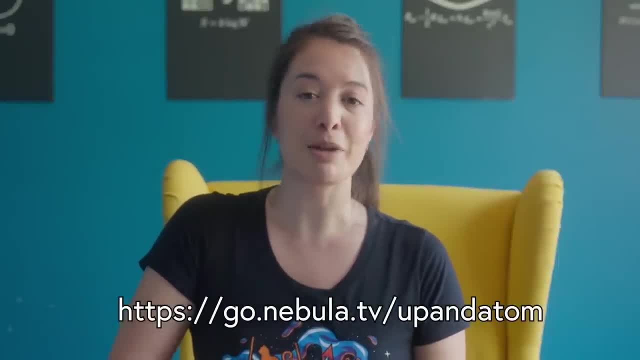 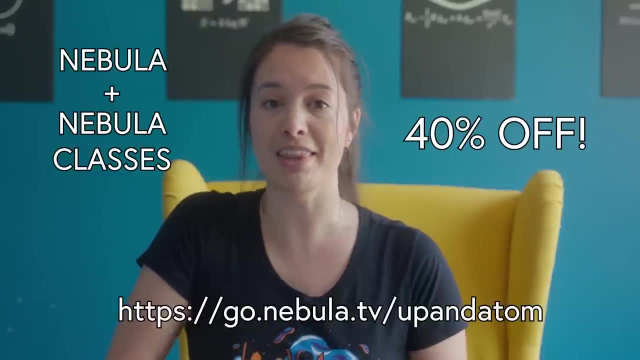 If you sign up using the link below, you can support me directly and get both Nebula and Nebula classes for 40% off the annual plan- As little as just over $2.50 a month. Thanks for joining me today and I'll see you in the next one.